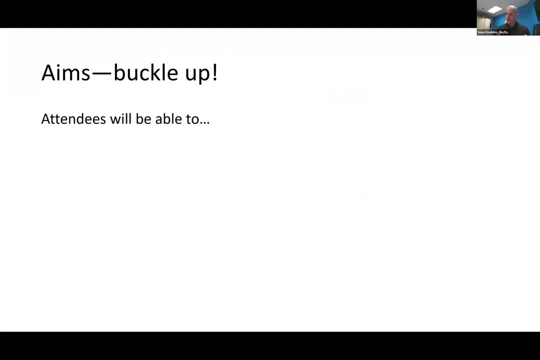 I really do hope that it transforms the way that you think about setting up and interpreting results from your experiments. What we're here to do today can be divided into four aims, but before we get started, I wanna lay out some norms for this talk. 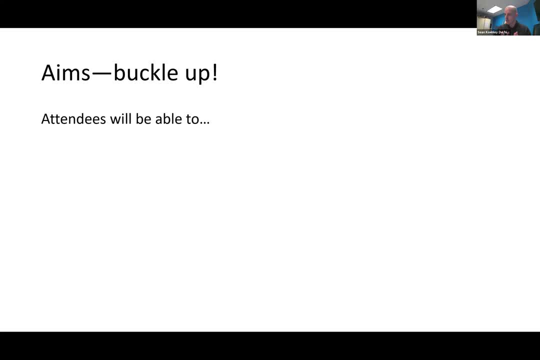 I wanna say that you can feel free to interrupt if you've got kind of a pressing question or some clarity to point. You can also enter questions in the chat. I probably won't see those until the end of the presentation, but there will be some time hopefully. 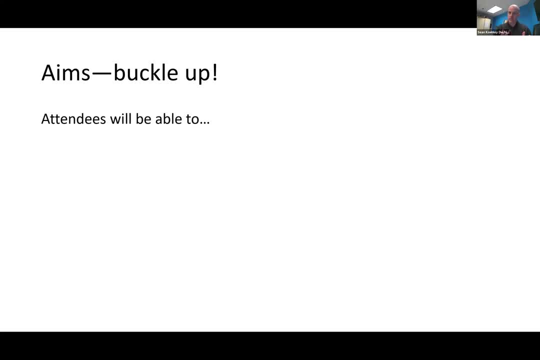 to answer some questions. This presentation is going to be recorded. I've got some extra materials for you as well, So any code you see, you'll be able to pick through and dig through on your own. I tried to make it as step-by-step as possible. I really do want it to be something that you can take and use on your. 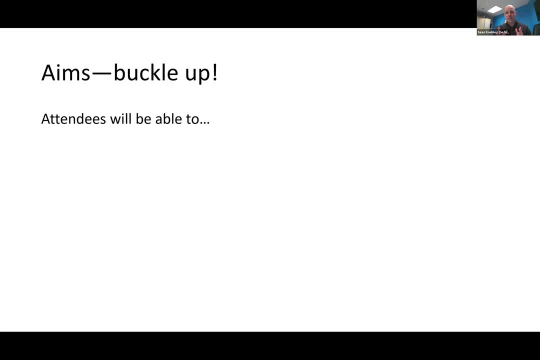 own. I do want to give a warning that there will be some math and some math symbols, just a little bit, maybe just a little bit of algebra. But I don't want you to get too overwhelmed. We're going to do it together And I just want to let you know that if you get lost, you don't get 100%. 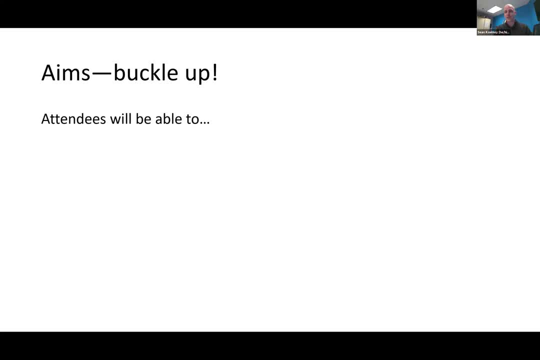 of this don't feel, don't just check out or feel like this is not for you, Because you know it took me a few times to get this And we're really just going for broad strokes today, introducing some vocab and letting you kind of see what this process can do. So any questions before we get? 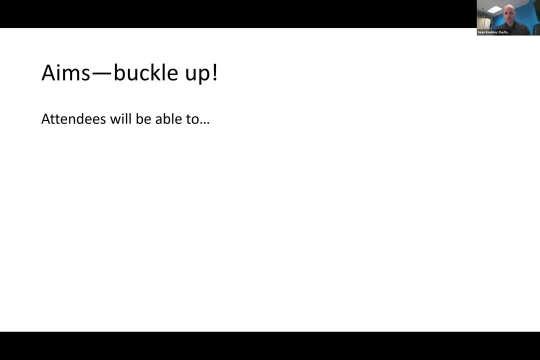 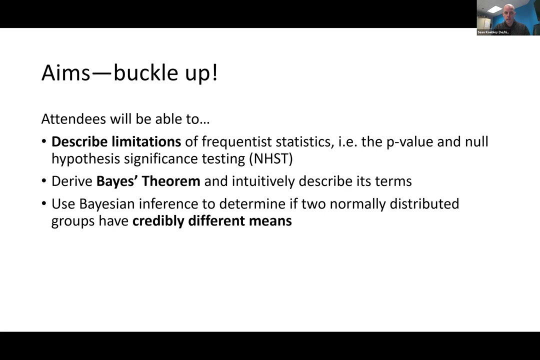 started Okay. So our aims today are: first, we're going to describe some limitations of frequentist statistics, or the p-value and null hypothesis significance testing, And then we're going to derive Bayes' theorem and intuitively describe its terms. We're going to use Bayesian inference to determine if two normally 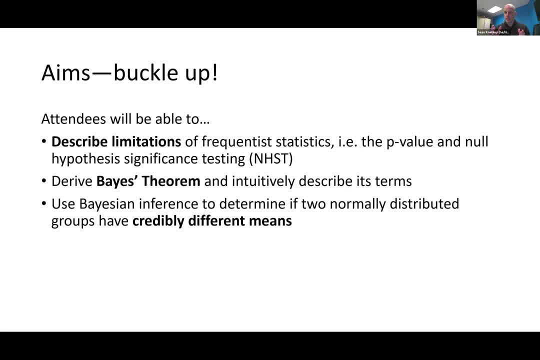 distributed groups have credibly different means. This is kind of the classic or one of the classic uses of the p-value. I want to see how Bayesian inference can do with that And throughout the talk we're going to be referencing useful resources for practicing frequentist. 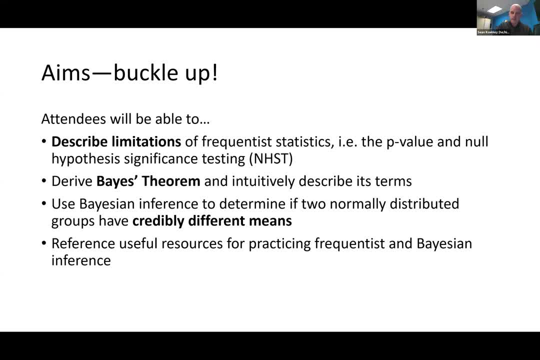 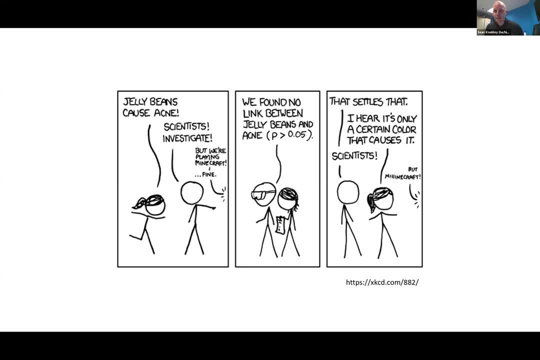 and Bayesian inference. So first we're going to start with describing some limitations of frequentist statistics. And here's a comic from XKCD. Maybe you've seen it before. It's one of my favorites. but you've got some aspiring researcher perhaps, or someone who's got this. 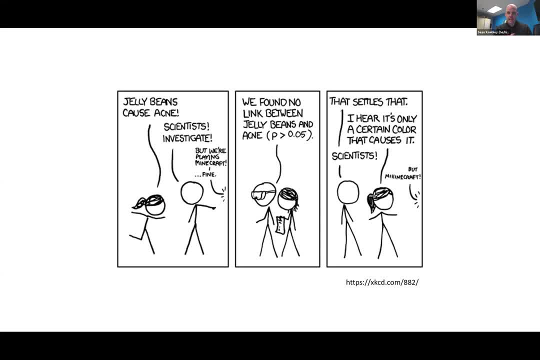 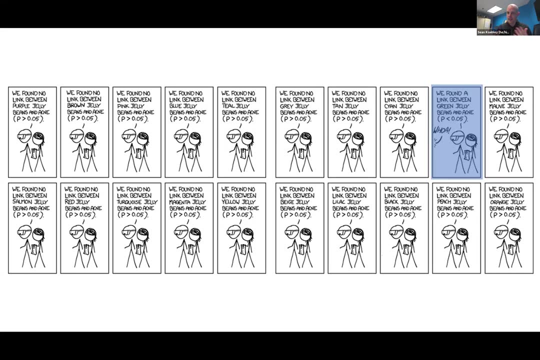 pressing question: thinking that jellybeans cause acne And the science is that jellybeans cause acne. So the scientists check it out and find no link. But the person in the question says that they think it's only one color. So the scientists try a bunch of different colors. In fact. 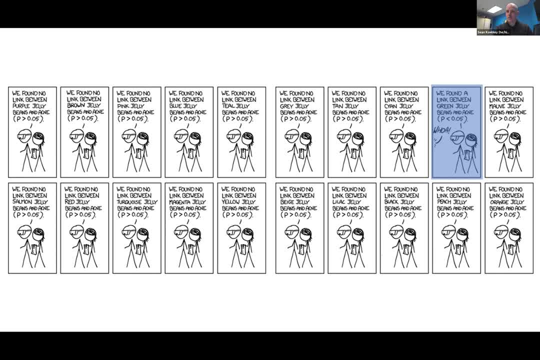 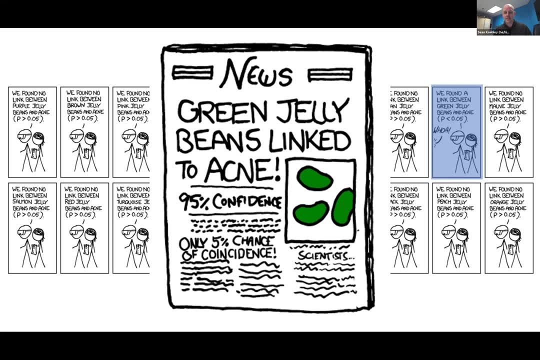 they try 20 different colors to jellybeans And in one of those cases, the green jellybeans. what do you know? They find a significant result. And so this is this crazy, you know, incredible result: that jellybeans, green jellybeans, are linked to acne. 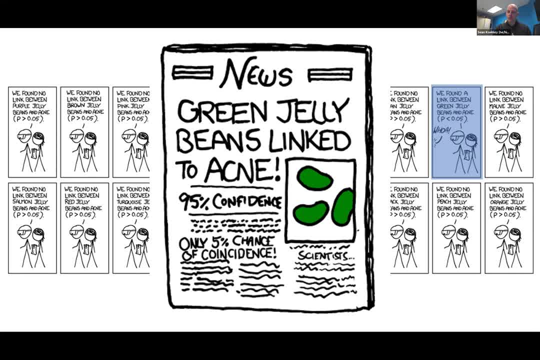 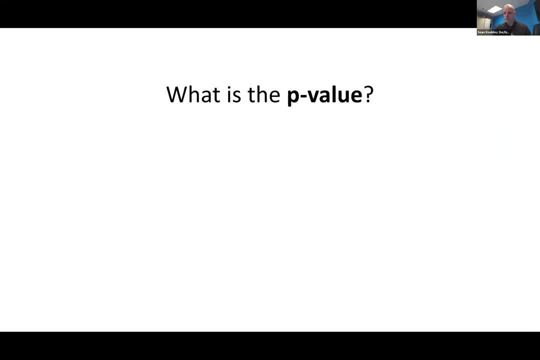 And, of course, this is kind of ridiculous And it's set up with, or this is a result of the way that we interpret, or misinterpret the p-value. So just want you to take some time right now. By the way, if you don't have a piece of paper or a pen, I think it's going to be very useful. 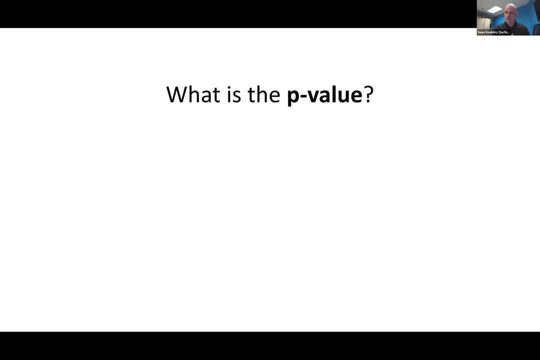 during this talk to have at least one or two pieces of paper So you can follow along with some of this stuff. But I want you to take maybe 30 seconds right now and write down what you think, your definition, what the definition of the p-value is. 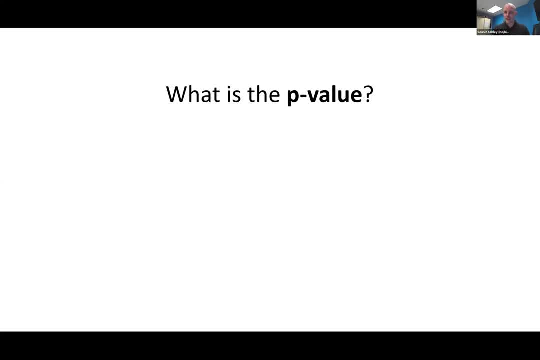 See if you can do it without Google. See if you can just do it off the top of your head And no worries if you don't get it 100% right. I'm just gonna give you about 10 more seconds. Okay, Do we have any brave volunteers? Does someone want to give this a shot? 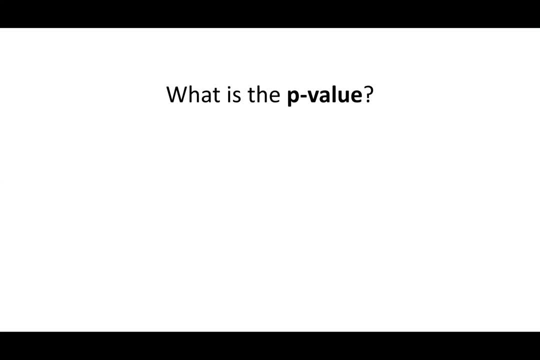 Do you want to give this a shot? Yeah, I'll try. Yeah, Yeah, Yeah Yeah, P-value is the statistical value that is used in relation to an alpha value in order to reject all assets and hypotheses. Okay, Yeah, So you're using a statistical value to reject, or did you say reject or accept? 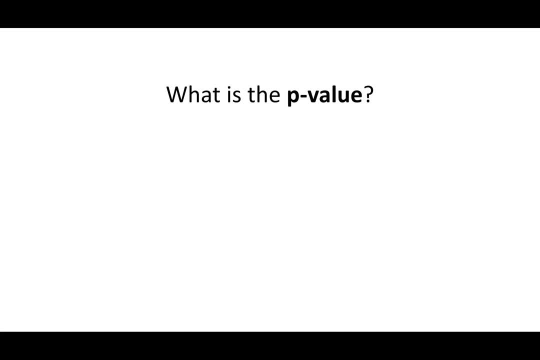 the null hypothesis, Yes, Okay, Yeah, It's close. It's kind of hitting around the borders. I think you've got some of the main ideas I will say. one issue with that is that actually the P-value is not telling you whether or not you can, or it's not a value of whether you can accept the. 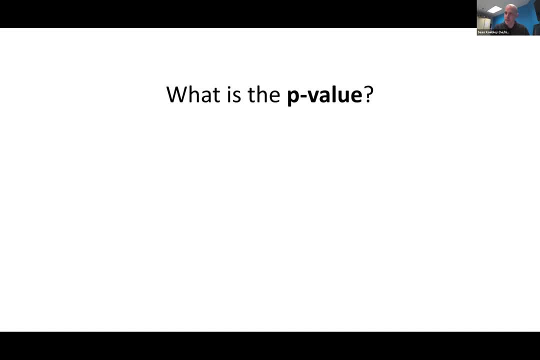 null hypothesis. It's only telling you whether you can reject the null hypothesis. So, yeah, Thank you, No worries. Yeah, And there's a lot. Yeah, Well, we'll see. It's not easy to get this whole definition right. Anybody else? I have one that I'm willing to volunteer. 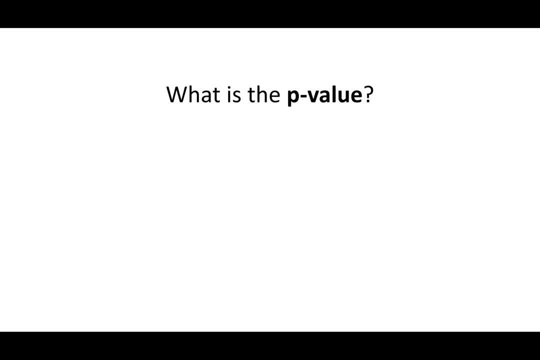 Sure P-value or the P-value, The odds that in a normally distributed population the difference that you see between the groups occurred by chance. I'm glad you said that And that's maybe what that's one of the main kind of misinterpretations that we might have with the P-value: It's not actually giving. 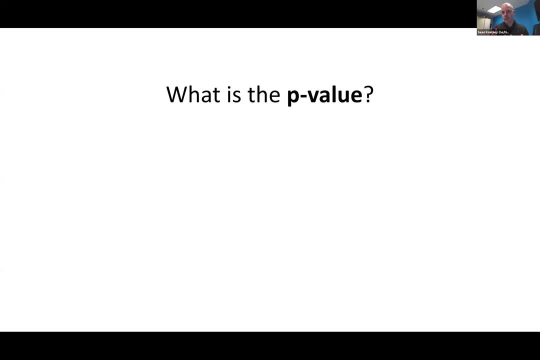 a probability that two things would happen by chance. I know that's kind of what it seems like, what it should be. It's not really what it's saying, but that's. I mean again, you're not alone. That's what a lot of people and that's what I think you know a lot of us believe what. 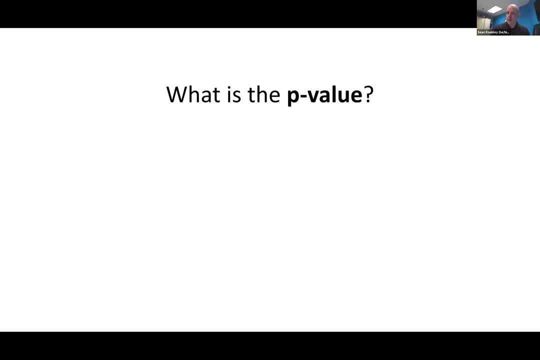 this is because that is the most intuitive interpretation of what you know. the results are when we do a statistical test. Anybody else want to give one more try? Can I try? Sure, So it's the probability, given that the null hypothesis is true, that you will observe a value. 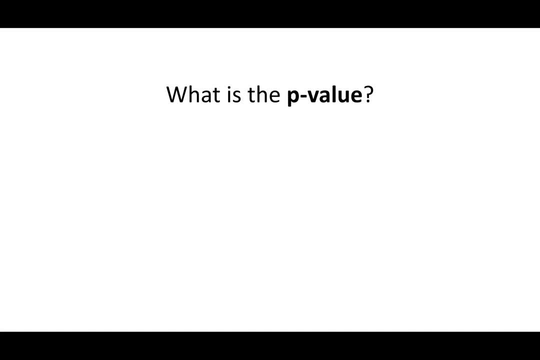 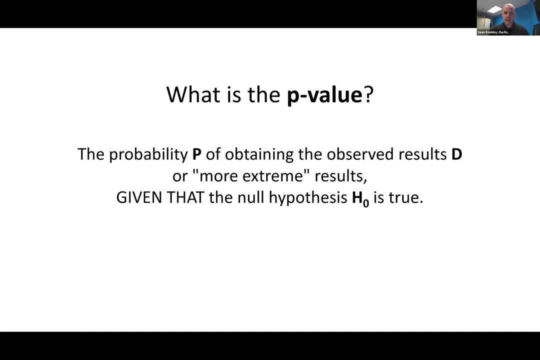 think you know I want to get across here is: the P-value is the probability of obtaining an observed result or more extreme results, depending on how you conducted the test, Given that the null hypothesis is true. So in math language or math terms, this is how we would write this. We'd say: 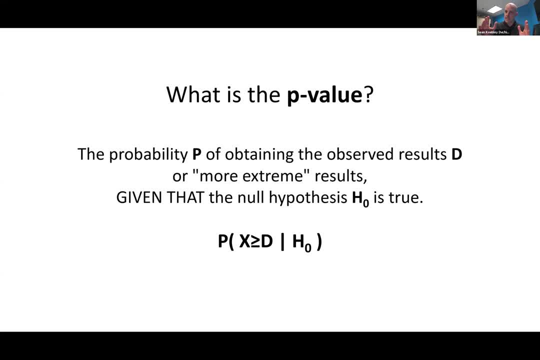 that it's the P of the probability of obtaining an observed result or more extreme results. but if you're looking at the probability of everything that's in the parentheses, your result, or X, is greater than or equal to the data that you observed. 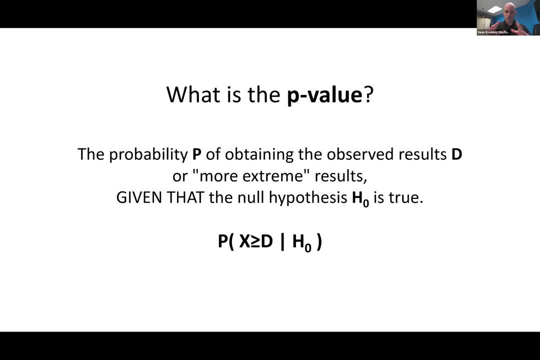 So it's, or sorry, so the X. so that's the probability of getting some result X. that's greater than or equal to the data you observed, something more extreme than the data you observed, Given that- that's what that straight line is, that means, given that the null hypothesis is true. 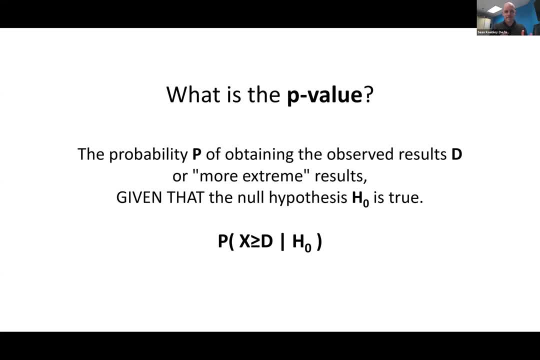 So again, very specific, Yeah, and maybe a little unintuitive, not really what you're thinking when you get some results from a statistical test and just want to put it out to you, maybe to see if anybody has some thoughts here, what do you think? is there another probability that would be more aligned with the goals of an? 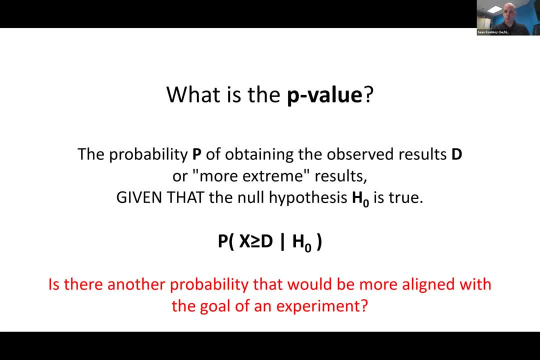 experiment. is there some other way that we could you know something else that we could try to get from our experiment that would be more aligned with what we're trying to actually discover? it's okay, I mean, and maybe what I'm looking for is something similar to what. 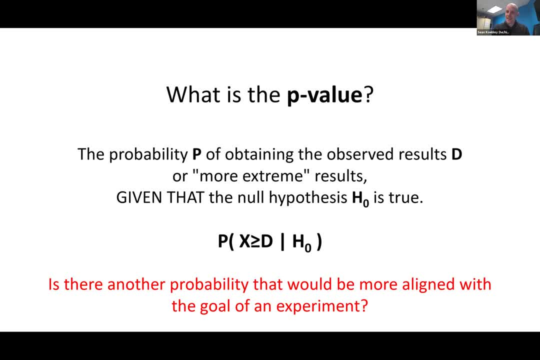 the first two volunteers said, which is again a more intuitive understanding of what we're looking for when we do an experiment. what about, okay, okay, okay. what about the probability that the hypothesis is true, given the data? right, right, exactly. that's kind of to me at least, and maybe you know, maybe to some of you, that's that's what I'm looking for. 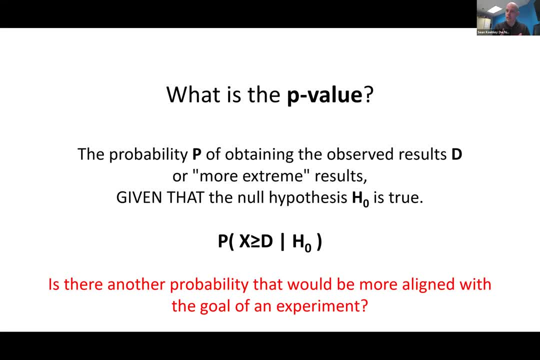 when I do an experiment I'm trying to find the probability of the hypothesis is true, given the data right. it's kind of a switch of what we're seeing written down right. here you're trying to find the probability that whatever parameters you're looking at have to be true, given that. 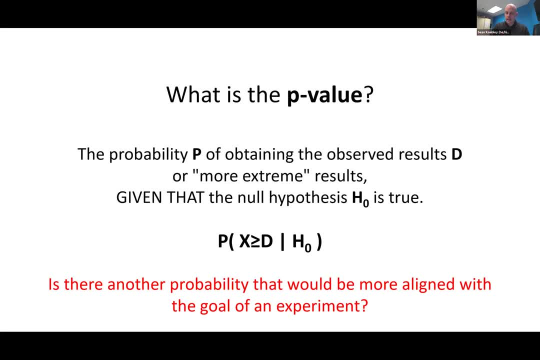 you're seeing the data. that's going to be true, given the data that's going to be true, given the that you that you observed. I know it's we're get. we'll get back to that later, But that's actually exactly what you're finding with Benjamin's statistics. 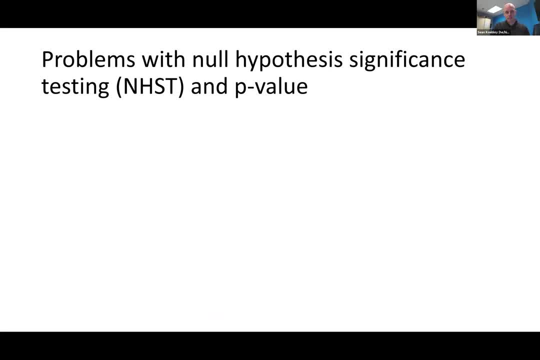 So just keep that, keep that in mind as we go through this. I just want to lay out some real quickly, some of the other issues that you can see with null hypothesis significance testing in the p-value. the one that we just kind of, I think, explored there is that it can be confusing and intuitive. gratitude. 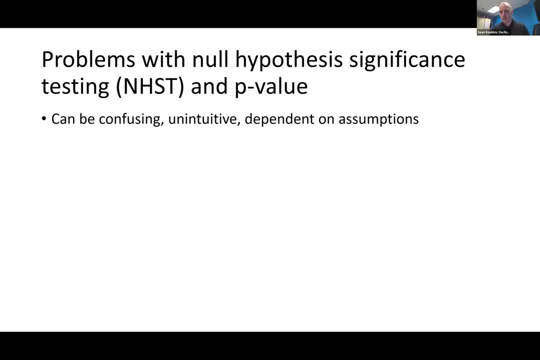 uitoitive input. Go to Sarada task, task of both the hand values that you use to convert. and also I'm gonna throw in there, dependent on assumptions. I know, when we shatter the polling figures, a loopatif driving guessing지는 questions. I know any of us who've done a null hypothesis significance test know that you have. 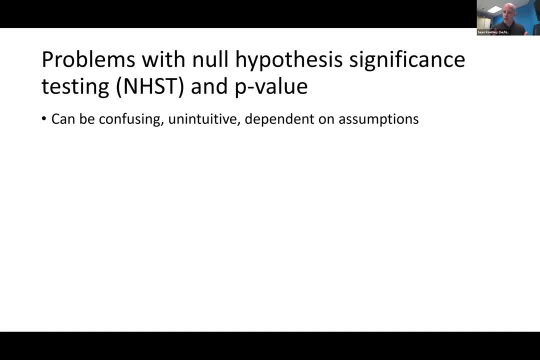 to. in a lot of the classic tests you have to assume normality in your data, which you know. there's additional tests you can do to try to see if that's true with your data, to see if they're actually normally distributed. But if they're not normally distributed, then you have to do a bunch. 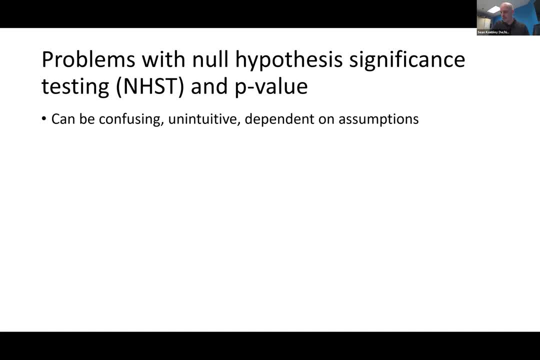 of other stuff. So it's just it's. you know it's complicated and perhaps needlessly complicated, given that there might be some other options out there. This is one that I think a lot of us are aware of as well. The p-value is dependent on sample size, So this can give rise to what's. 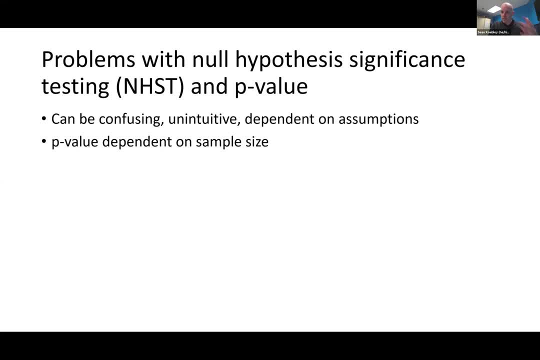 known as p-hacking, where you, you know, take a bunch of samples. you don't get the result you want. perhaps This is some nefarious research of doing this. I know none of us would ever do this- but you don't get the result you want. and then you do. you know twice as many. 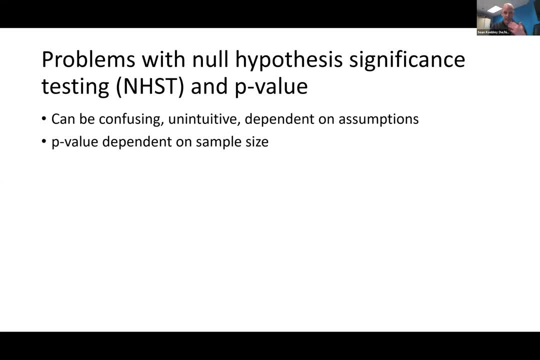 um experiments and then suddenly your p-value is below 0.05.. And so then you stop Um. so that's, that's kind of these, and because it's just a single value, there's no other kind of uh. 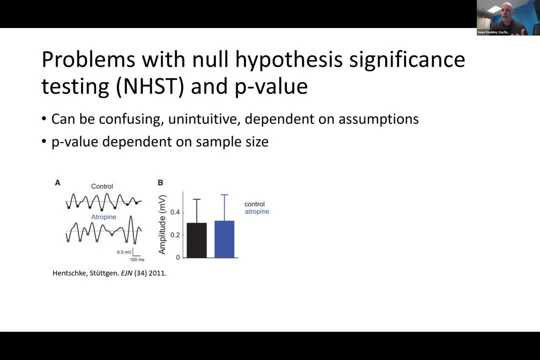 interpretation or or additional context for a p-value? Uh it's. it can be difficult to see where that n comes in or or what the reference is for that, So here's just a quick example of this uh from this paper from 2011.. If you're trying to test the effect of a drug, uh. 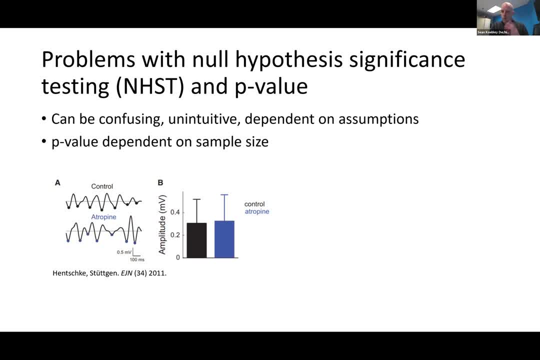 actually, you're going to have to do a lot of research. You're going to have to do a lot of on a control. Uh, what we're going to see here is just um mapping that effect, uh, as we take. 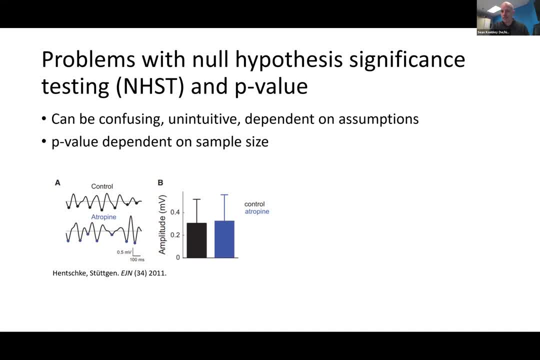 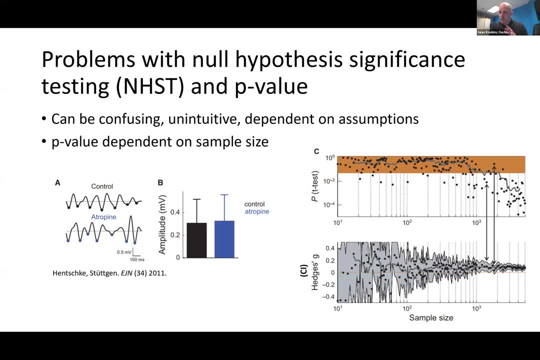 more and more, more and more samples. So if you just take 10 samples, the difference between the means looks negligible. They look very similar, And so what I'm plotting here is, on the top, the p-value. uh, if, if you do a p, a p-value between, uh, comparison between these two. 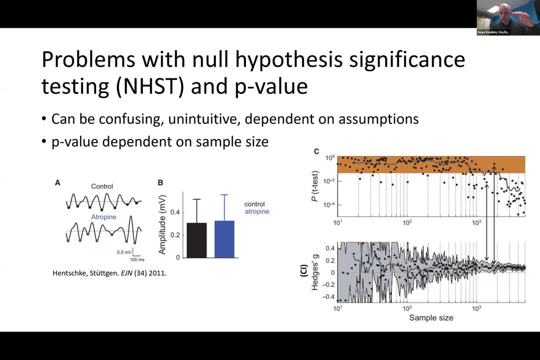 uh groups and you can. and if it's, you can see that magic number of 0.05, is is uh, anything below the orange. So all those tests that you see when your sample size is very low are, you know, mostly above the orange. So as you get through, um, you know. 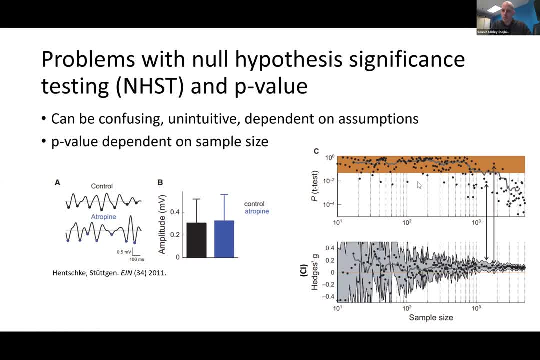 past. but then, as you, as you get to more and more samples, you see your p-value dip below that orange um line, which means you're getting significant results. all of a sudden, uh, once you get, you know, over a thousand samples, uh, now, below the plot, below you can see: 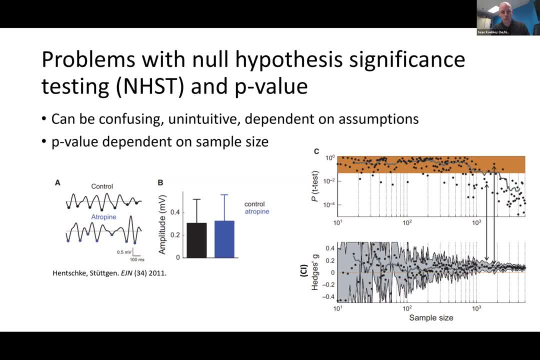 uh, the hedge is a G or one of or uh one, one way of of calculating the confidence interval, And it looks a little different and maybe more useful. Um, you can see it's starting out very wide, meaning that there's a lot of uncertainty as to what the actual effect of the drug is. 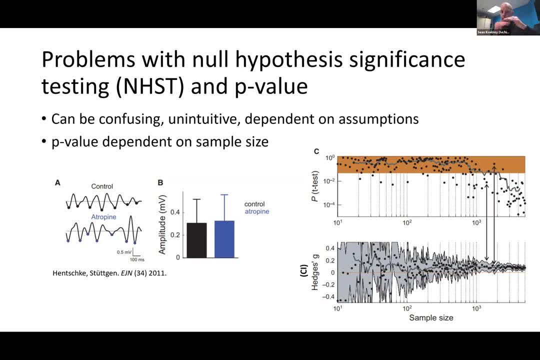 And then, as you get more and more samples, you can see that confidence interval narrowing Um. so you're, and it's, it's, above zero. So you're seeing that significant result, which means you're seeing some effect that you can assume with confidence is more than zero. 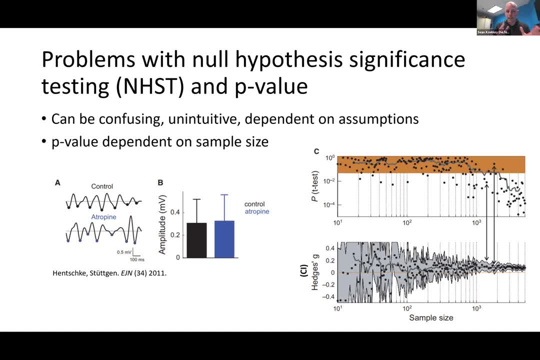 Um, but it gives you more context. basically- And that's one of the lessons maybe that I'm sure I'm sure many of us know, but I want to reinforce here- is is that the confidence interval is is better than the p-value, gives you more context. still has some issues, though. 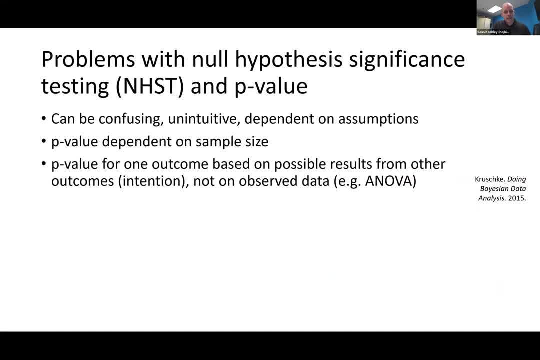 Um, another kind of weakness of the p-value is that it's one outcome based on the, the possible results from other outcomes, uh, the intention, Uh. so there's this whole cloud of possible intent of outcomes that you, that is implicit when you read a p-value. it's not really based on the observed. 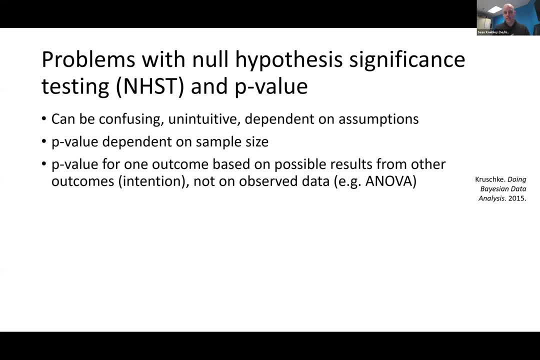 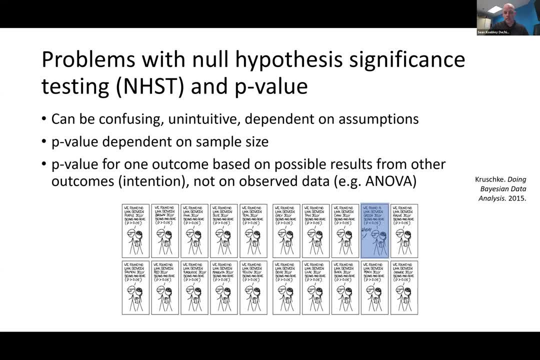 data, which is is a bit of a complicated concept, but I think the one that kind of drives it home for me is is an ANOVA test. if you get a situation like this, where you get a p-value of 0.05, less than 0.05, well you know, it doesn't really make sense to base your p-value just on that single. 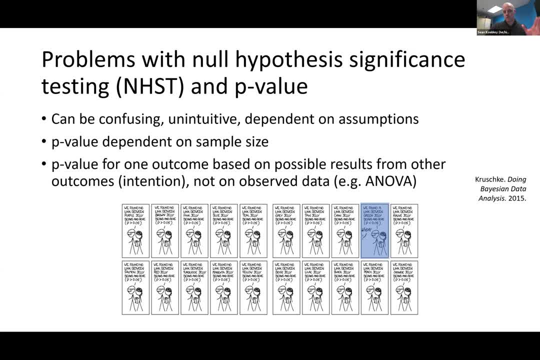 test, because your testing intentions included the sphere of all those possibilities, all those different colors that you were testing. so in ANOVA, you have to be very careful about this. you have to adjust, you have to apply some normalization factors and really be careful about how you. 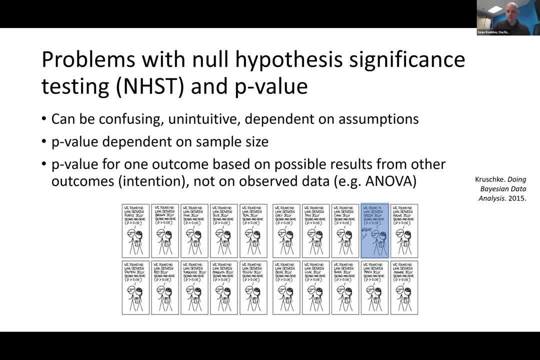 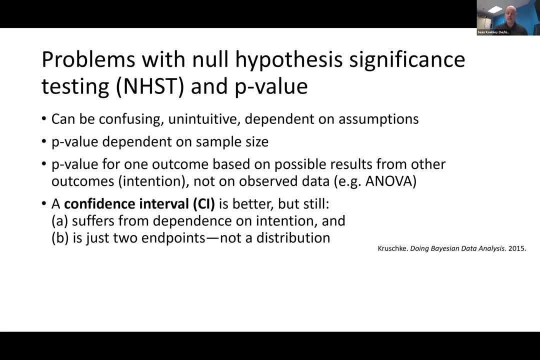 interpret those results because of this exact effect. so one way to kind of enhance your null hypothesis, hypothesis significance testing is to use a confidence interval instead of, or in addition to, a p-value- definitely a good idea, and I'll give you a resource, if you're not aware of it, in just a second. that's my favorite. 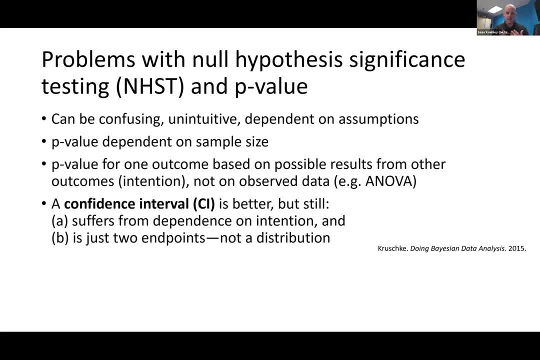 for kind of dealing with null hypothesis, hypothesis significance testing. but I'll say that the confidence interval still suffers from a dependence on intention and it's just two endpoints. it's not actually giving you a distribution of where the most likely values for a mean say might be. so when 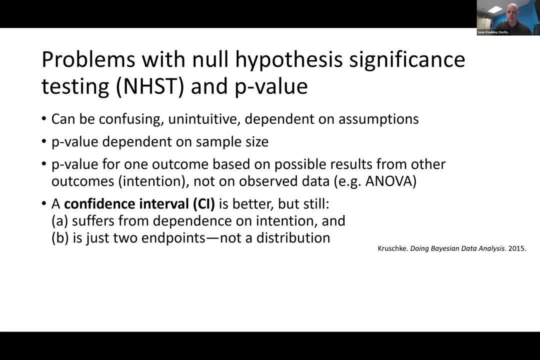 you see a confidence interval you're just seeing two endpoints, also not as great as you might want. so this is one of the main kind of weaknesses of null hypothesis significance testing. that I think, is kind of kind of shocking in some ways if you look at certain examples. so, for instance, if I'm looking at a fair coin, I'm trying to see if a coin is fair and I run a bunch of experiments to determine that by flipping a coin. what would my null hypothesis be in this case? 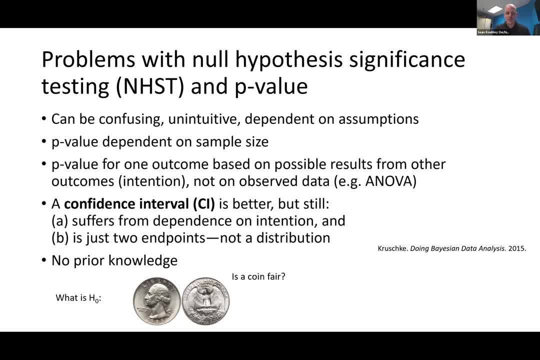 anybody want to volunteer? that's my null hypothesis. if you're trying to test to see if a coin is fair, that the coin's not fair, um, well, I think. well, that's um. well, actually I'm looking for, like, maybe a- sorry, maybe I was unclear about this link- for maybe like a number, so what's so? what percentage of um your, your flips? 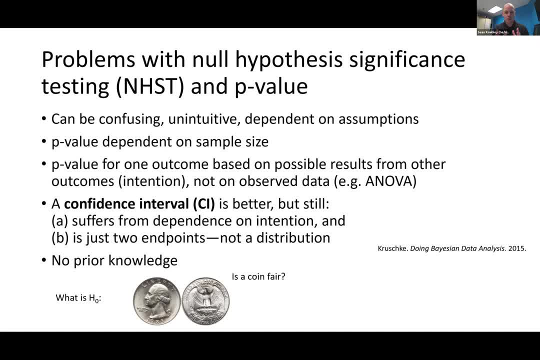 did you expect to be heads, so sorry, so maybe that would be a null hypothesis. is there a way that you could use that? so I'm just saying what's yeah if I'm looking at the number of yeah, zero difference: 50, 50, yeah, 50, 50, sorry so yes, so your null hypothesis in this case would be: 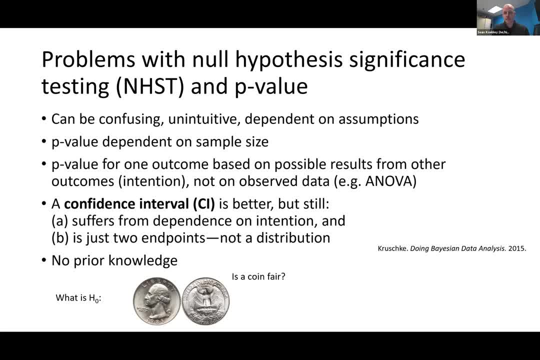 that, um, the chance of getting heads is 50 or 0.5. now what if we're testing a nail? we're seeing what if the what's the chances of getting heads when you flip a nail, where heads means the nail, you're not going to be able to flip a nail. you're not going to be able to flip a nail. 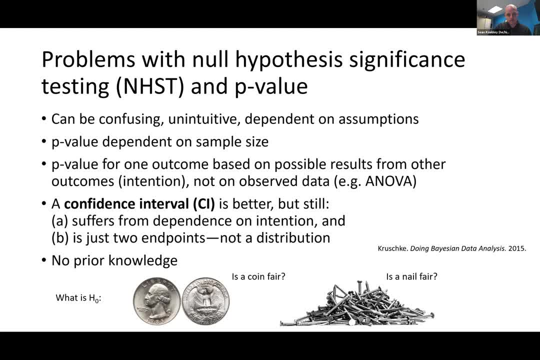 lands directly on the head of the nail. so if we're asking if the nail is fair, we actually have to use the same null hypothesis. this is the crazy thing about testing null hypothesis, uh, significance testing. you have to. you know, if you're trying to disprove your null hypothesis, you have to. 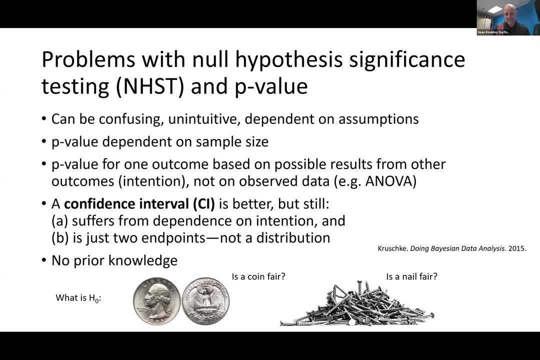 you know, use that null hypothesis. so it's actually the same null hypothesis that the chances are 50- 50 that you're going to land on heads. and again, this is maybe a weakness that you might have seen in some of the literature: people testing null hypotheses that have no chance of being true, so they might test. you might say: 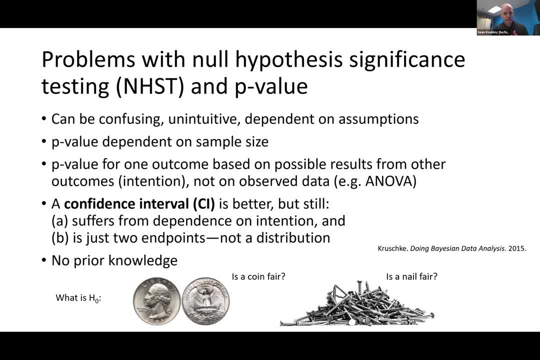 all right, this drug has no effect. well, you know, we can be pretty sure that if it's a drug that's an iteration of a previous drug, it has some kind of effect. so that that's what I mean. it can be really really difficult or doesn't make a lot of sense to assume a null hypothesis that a nail is. 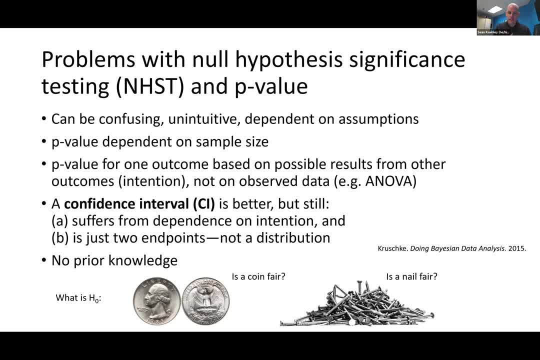 fair or that a drug has no effect, when you know it's pretty clear that the nail is not fair or that there isn't some effect. so what? the way we you know- I want to put this in terms of this: saying there's no prior knowledge, that we have when we there's no prior knowledge built into a null. 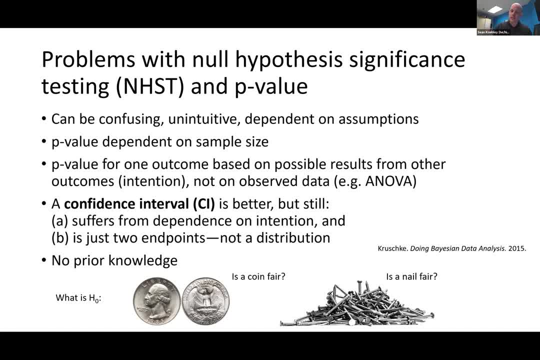 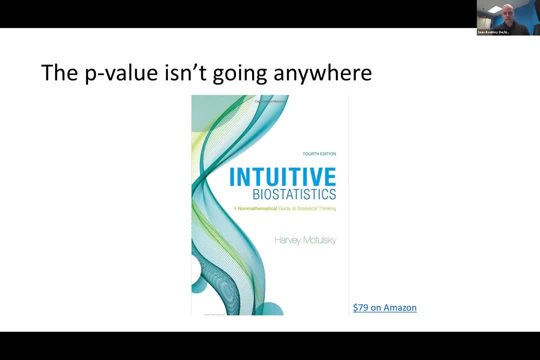 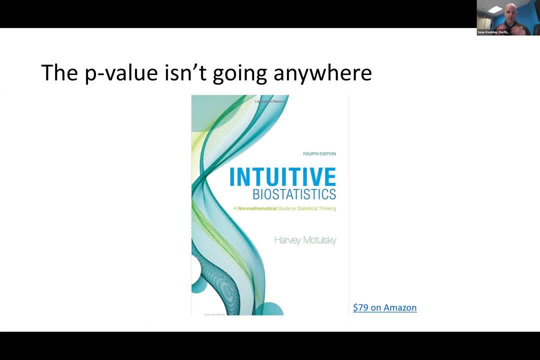 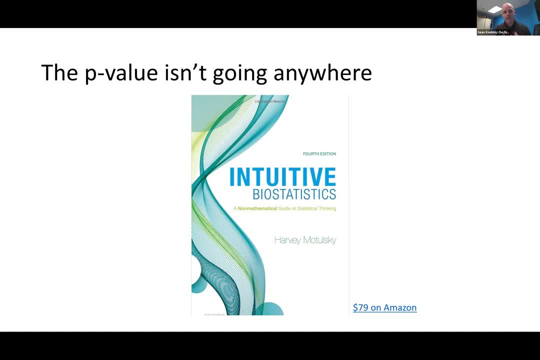 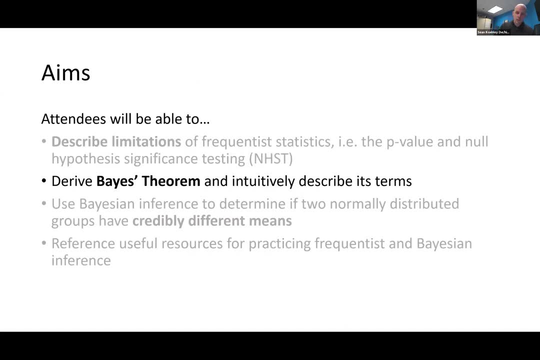 an amazing intuitive look. very little math, a lot, of, a lot of intuitive explanations, so I highly recommend it. moving on to our next aim, we're going to derive now Bayes theorem and intuitively describe its terms. so we're going to get started with what Bayesian statistics are going to be. 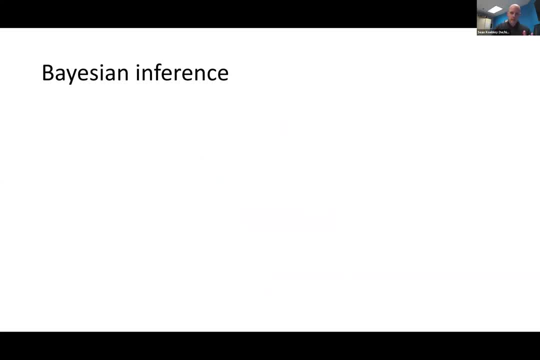 and we're going to get started with what Bayesian statistics are going to be and how we can use it. so just a little, a brief, brief background. Bayesian inference has actually been around before null hypothesis significance testing. it came about in the 1700s. Thomas Bayes was an English mathematician, so it's been around before. 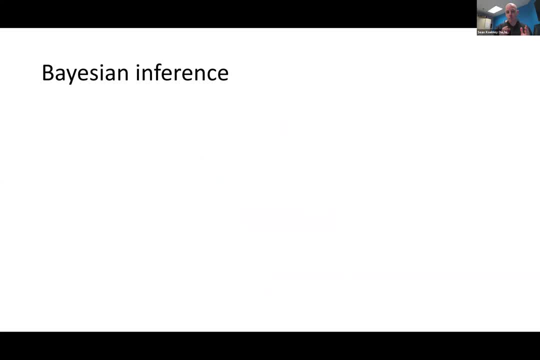 null hypothesis significance testing, but it wasn't as widely used for one major reason that we're going to get to in a second. it had one major flaw: that that made this other technique of the p-value come the preeminence. so, Bayesian inference, as simply as I can state it, is the reallocation of credibility towards parameter values, theta. 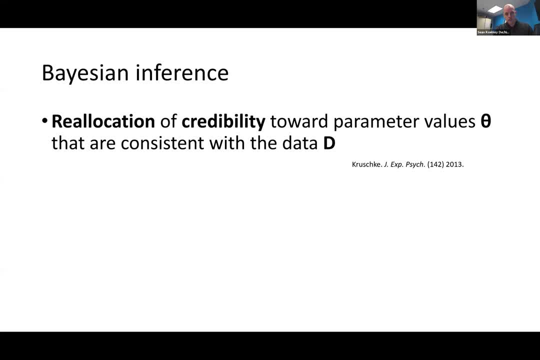 that are consistent with the data d? okay. so that may seem like like a mouthful, we're going to break this down. okay, when we say a reallocation of credibility, you're starting with your prior knowledge. okay, and what's great about Bayesian statistics is that you're going to be able to. 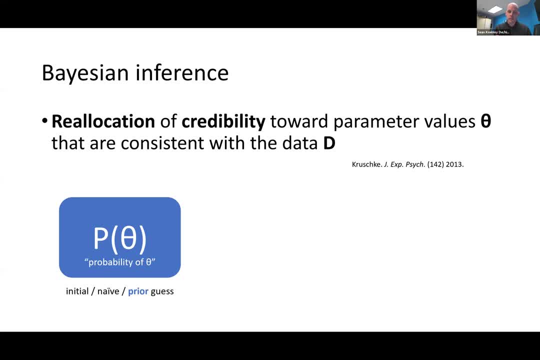 be extremely explicit with how you define your prior knowledge, what exactly you expect your parameters to be okay. so when we talk about a prior knowledge in Bayesian statistics, we're actually talking about this value here, the probability of theta, or the probability of your parameters being true, a certain set of parameters being true. so this is an initial 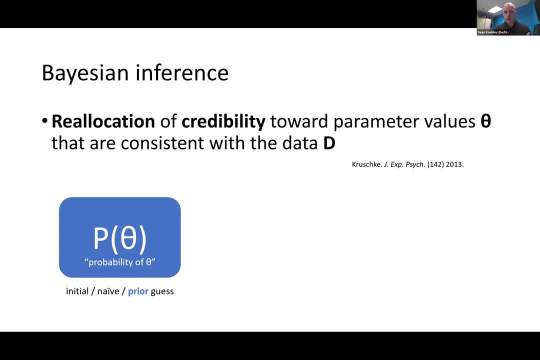 a naive or um. you know it can be informed by pre, by prior data as well, so you might have some preliminary results. you might have some preliminary results. you might have some preliminary results that give you some idea of what theta should be, and this is your prior knowledge. then you refine. 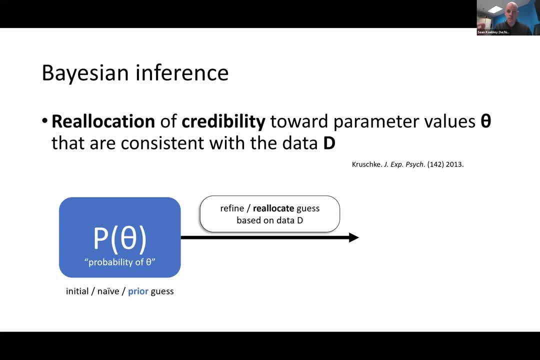 or you reallocate your guess or your knowledge based on the data d to get your posterior probability or the probability of your parameter values, theta- being true, given that you've collected the data that you've collected. so, again, this is a much more intuitive desired endpoint of experimental. 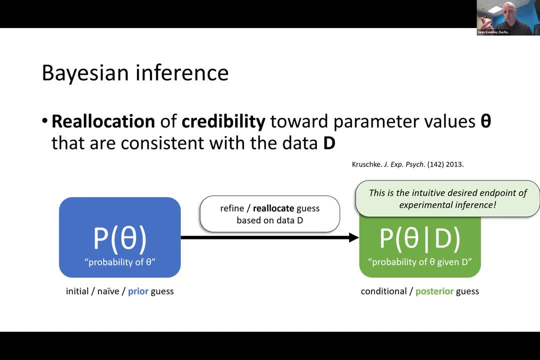 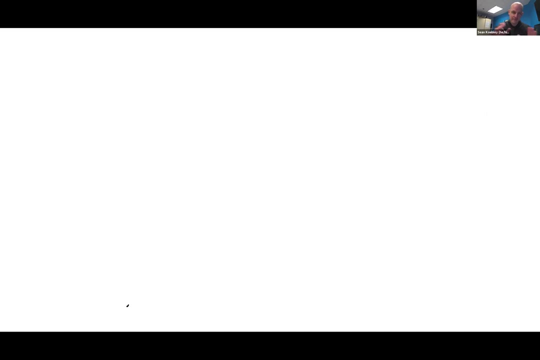 analysis and you're the one who gets the most information. you're the one who gets the most information and you're the one who gets the most, given a lot of data and so on, but in the case of a prior knowledge, you're the one who gets the mostレ. 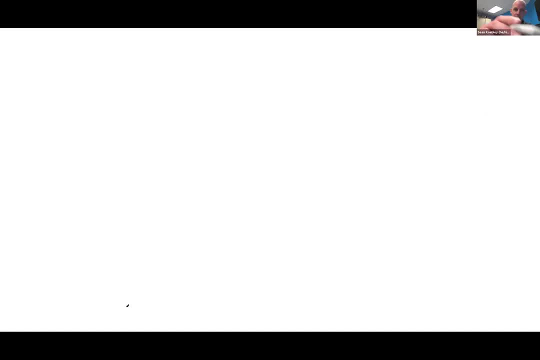 you're the one who gets the most data and you can see the difference in your params, in your parameters, And I think it's only fitting that we start with an example that might be on the minds of many, which is March Madness. We're going to do a March Madness example. 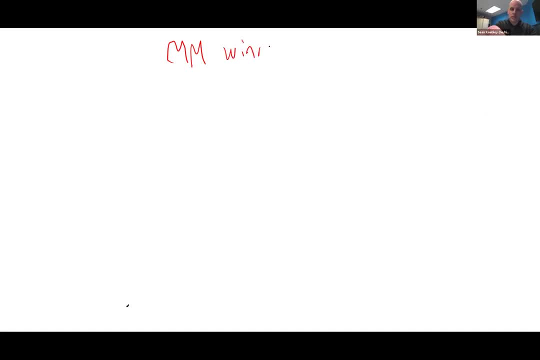 And we're going to do March Madness winners since 1979 is what we're going to work with here. Let's see if I can get black instead of red. So I apologize if my writing isn't the best here. I'm going to do my best. 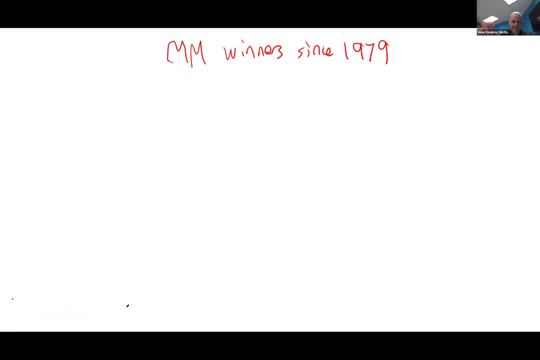 This is my wife's touch screen. It's going to be great. It's going to be great, Okay, so we're going to make a little table here, a three by two table, And our columns are going to be the seed of each winner. 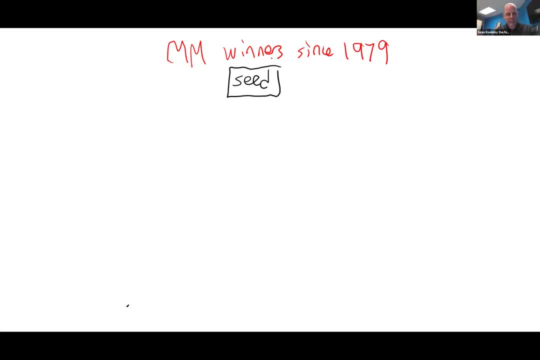 So, if you're not familiar with basketball or March Madness, the seed is like the ranking And there's actually four number one seeds every year, because each division or region or whatever gets their own number one seed. So we're going to divide this into two columns, whether you're a one seed or a greater than one seed. 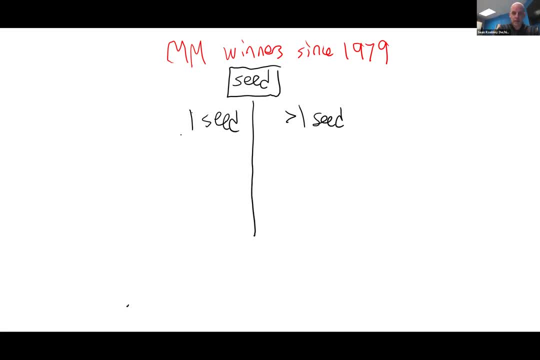 Just do that, Leave a little bit of space at the bottom there, And that's what we got. Okay, And then our rows are going to be our teams. Okay, We're going to do the two programs that have won the most championships since 1979, UNC and Duke. 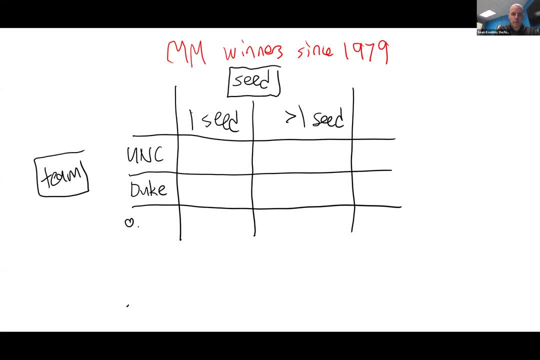 Five each, And then we're going to do everybody else. So we're making this table, because Bayesian statistics is dependent on count, It's dependent on conditional probability. This is a really nice, simple way of looking at conditional probability. And yeah, don't get too hung up on what these particular values are. 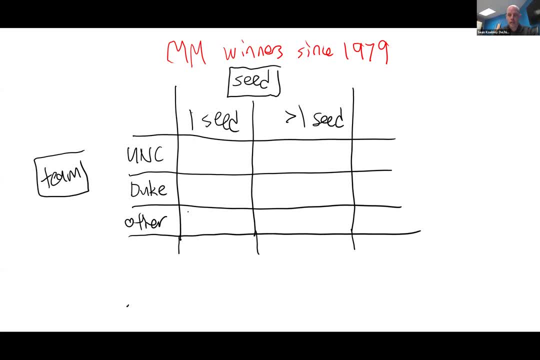 I want you to think about the logic that we're trying to build, And you know for that, for that purpose, we're going to call these seeds, or seed options, our parameters. Okay, Call those our parameters theta, And we're going to call our 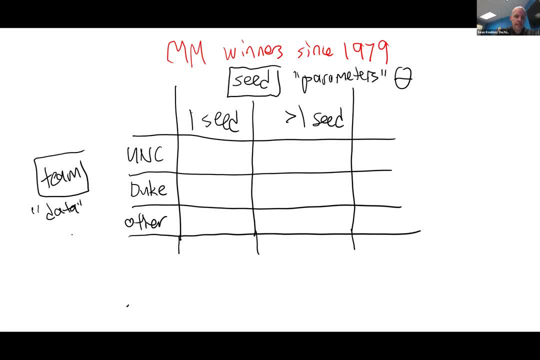 Our teams, our data, our data. D. Why did I choose the seed to be the parameters? No reason Could have been unswitched. I just want to start to get you used to thinking of the relationship between data and parameters. So we're going to call this number one, seed, theta one. 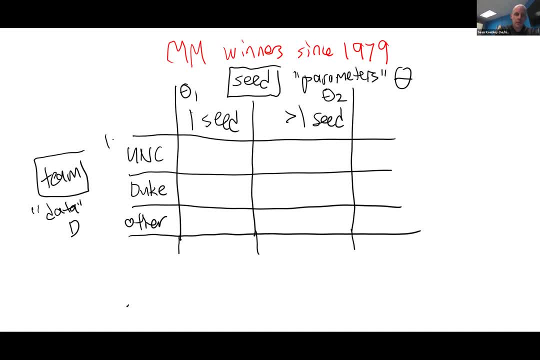 We're going to call this greater than one seed, theta two. UNC is going to be D1.. Duke is going to be D2.. And then other is going to be D3.. Okay, Okay, So let's fill in our table with some real data. 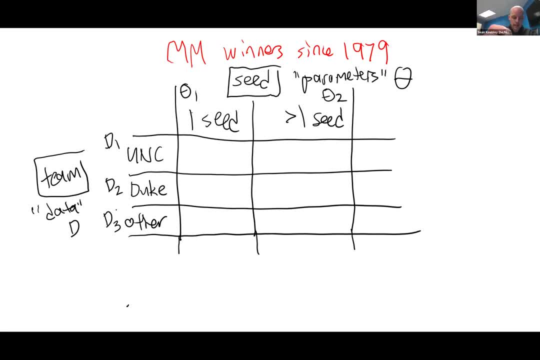 There's been 40 championships since 1979. And what I'm going to give you is the probability of UNC winning as the number one seed. That's what we're going to put in this little square right here. The probability is 0.125 based on that last 40 years. 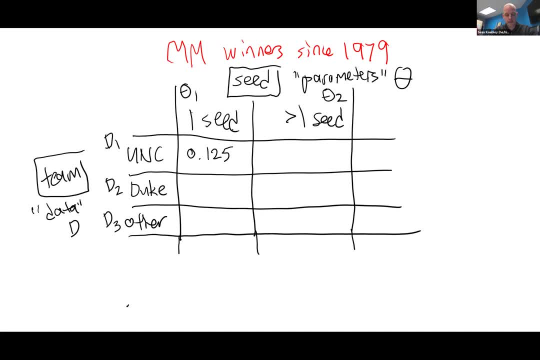 So those 40 championships, So I think that won five out of 40 when they were in, And that's a lot of times, And I think that's a lot of times. one of those times they were ranked the number one seed. So actually it's zero times that they. 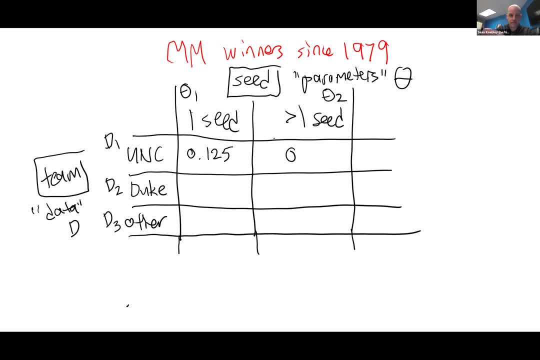 were not ranked the number one and also won the championship. So we're just going to fill in the rest of those values here. That should be 0.025.. Got 0.35. And that's it. So we're going to add to our table here. I'm going to start with our first kind of 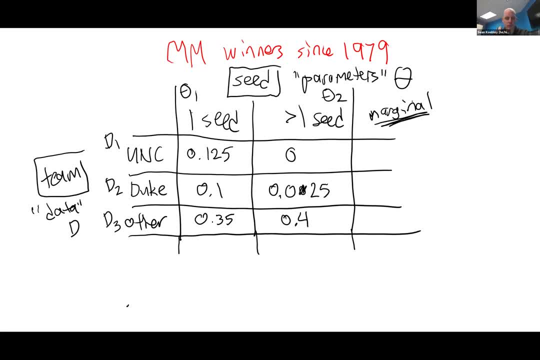 well, maybe not our first, but one of the major vocab terms that you'll come across- And sorry, that's an M for marginal, So we're going to describe our marginal data. Marginal just means unconditional, So there's no condition that's applied to this value. 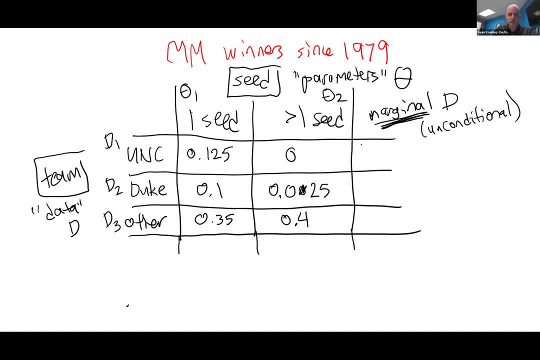 And how we're going to get that. we're just going to sum up all of the data in one row. So I'm going to get 0.125 by summing up 0.125.. I'm going to get the same for Duke when I sum. 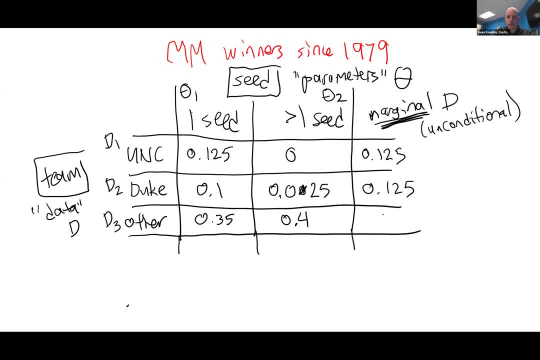 up everything in that row And then for everybody else we're going to get 0.75.. Now I also have marginal parameter values, And so I'm just going to sum every column: 0.575 is the chances that the winner was a number one seed, which is kind of interesting, I thought. 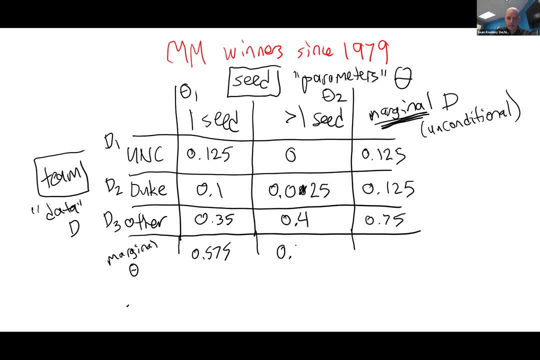 It's very likely that the winner of the tournament is a number one seed, And 0.425 is the chances that they weren't number one seed, So okay, So this is our table. We've defined marginal. Now let's ask some questions And 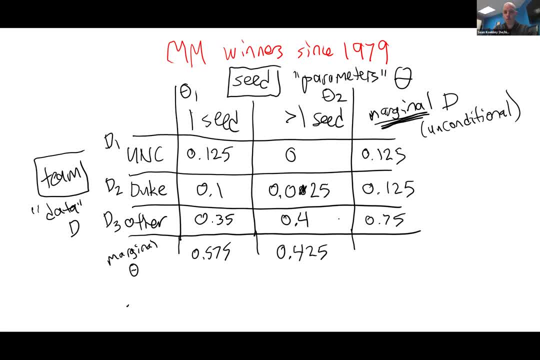 one of them might be. what's the probability that again a number one seed won the tournament? That's this value right here, Or p of theta one. So that's what we call the marginal probability of theta one being true, Or our prior knowledge. It's unconditional, There's no conditions. 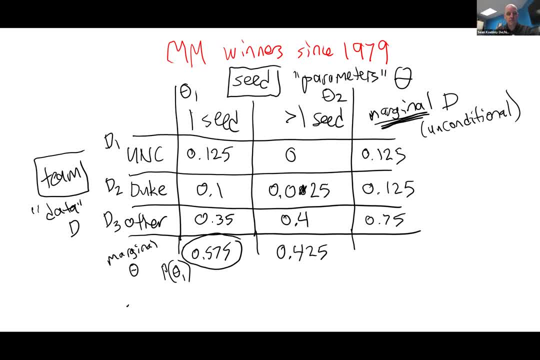 on this knowledge. It's just the probability of theta one. Now we can also have over here probability of d2.. That's the marginal data, Or the probability that Duke won a tournament. So that was relatively easy. Let's go on to a tougher one. Let's say what's the probability of? 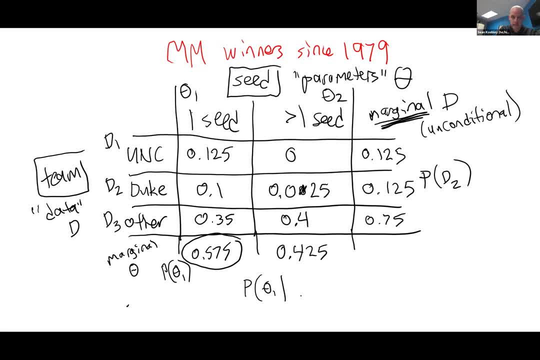 theta one given d2.. Or the way we'd say this is: what's the probability the winner was a number one seed, given that we know already that Duke was the winner? So we're only considering cases where Duke was the winner. What's the probability that the winner was a number one seed? 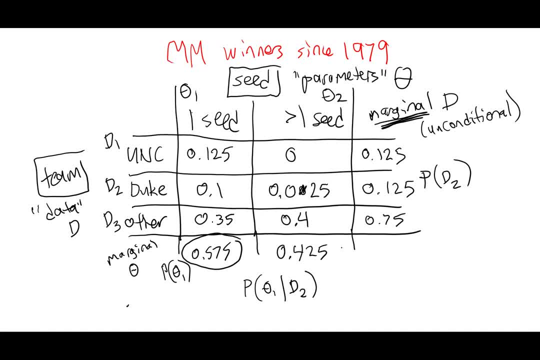 0.1.. It is not actually- And this is the here's where we've got to think about that given term. So we need, when we say, given that the winner was Duke, It means we're focusing only on this row, We're only focusing on the cases where Duke was the winner. 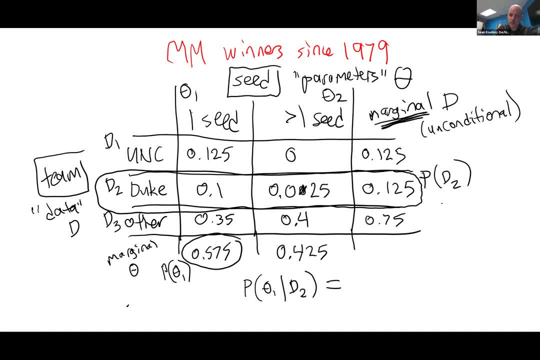 Okay. So I think this is this is really important. This is kind of the whole- and you'll see in this the definition of Bayesian statistics- What we do when we say, given that something is true, It's actually giving us a new focus, Or another term for that is we're reallocating. 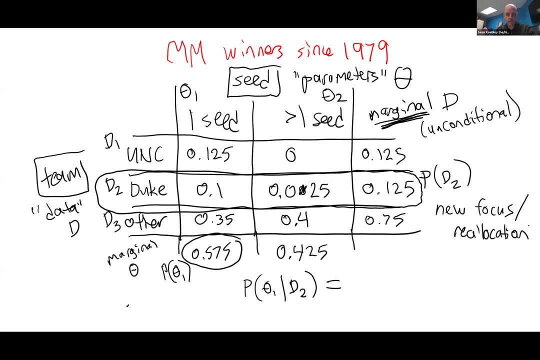 our probability. based on that, based on what's given to be true. So think about that. Think about that one more time. Given that, Duke is the winner, We're only looking at cases where Duke is the winner. We're focusing on that row. 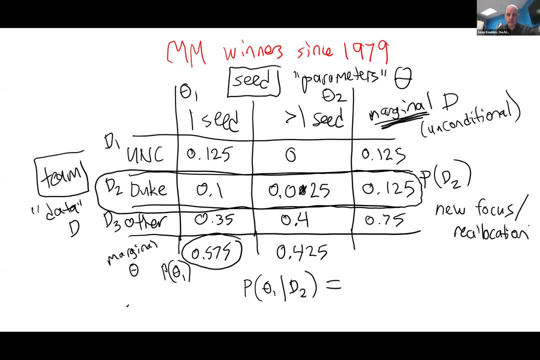 We want to look at the cases where the winner was a number one seed And Duke was the winner. Does anybody have any 0.8? then, Yes, that's it. Yeah, And if you, if we're not sure, we got 0.8.. We're looking at. 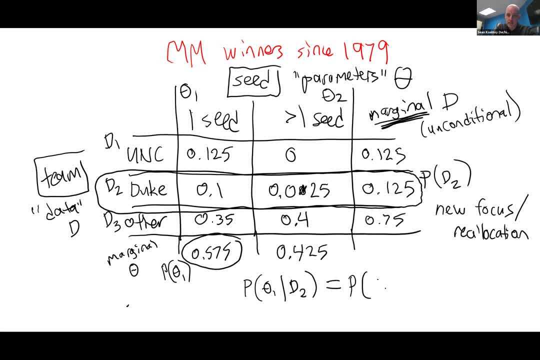 the probability that the winner was a number one seed And the winner was Duke. So that little comma means and Which is this term right here? We're dividing that by the probability that the winner was Duke. So again we got that new focus And hopefully this, if you again this may- maybe you're not 100%- 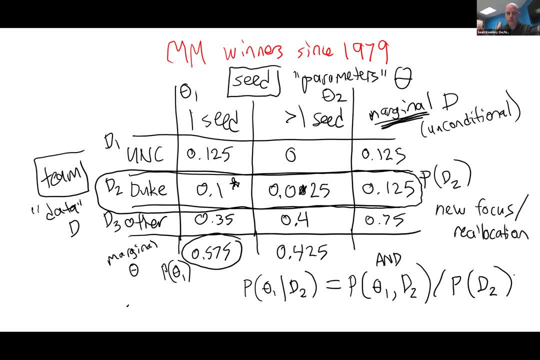 getting this. But think about it a few times, You know. maybe come back to this And see if that makes sense. Given that Duke is the winner, It means we're in this row, We're focusing on this row. What's the chances that the winner is a number one seed? It's this guy divided by your total, or your. 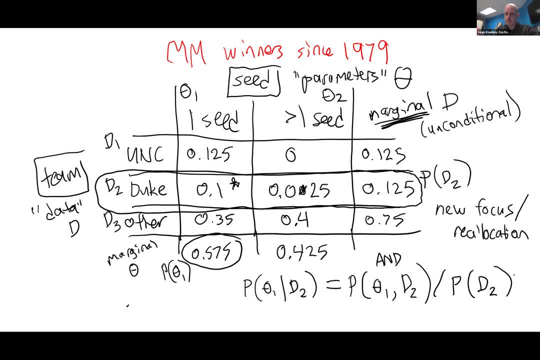 marginal value. So seems simple, But it's actually a very powerful concept, As we'll see in a second. But I want you guys to maybe try this one more time with a different question. We're going to flip it, Okay, given that, Let's try this instead, Given that the winner was Duke. 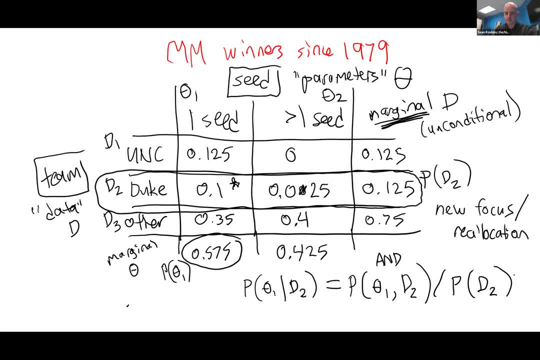 What is the probability that the winner was a number one seed. So say it again, Given that the winner was Duke, Maybe I'll write it off in this corner, Running out of space, Given that the winner was Duke. Sorry, given that the winner was the number one seed. 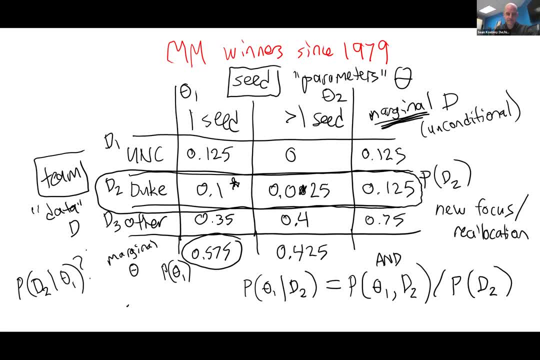 what's the probability that the winner was Duke? Maybe you don't have to calculate this exactly. you might need a calculator for it, But does anybody have the division problem that you would use here the numbers that you would plug in? Would it be 0.1 divided by 0.575?? 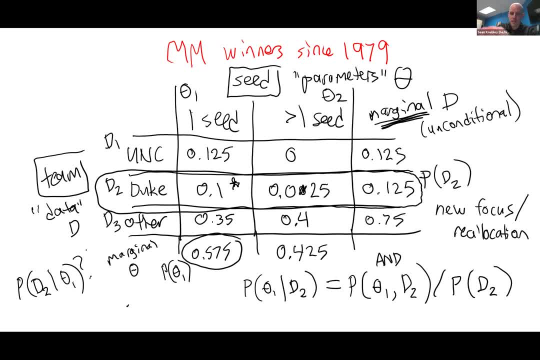 That's correct. This time, our focus is that first column, That's the reallocation, is based on the probability that the winner is the number one seed Cool Again, let's keep these concepts in mind and we're going to do some derivatives. 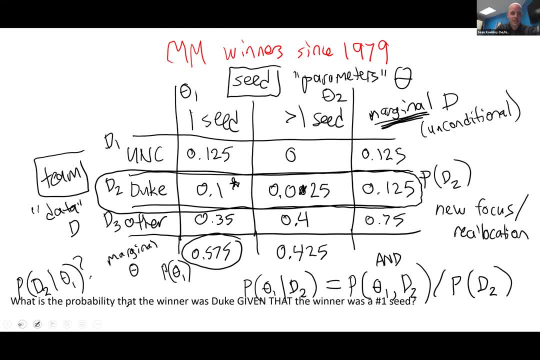 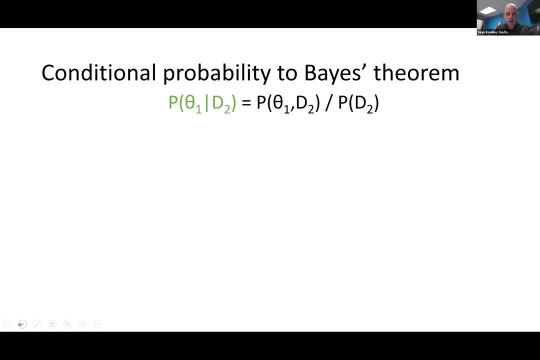 There's that question that I just asked. Again, this is recorded, so if you didn't quite get all that, it'll be on there. Here's what we just wrote down: Probability that the winner was the number one seed. given the probability that the winner was Duke. 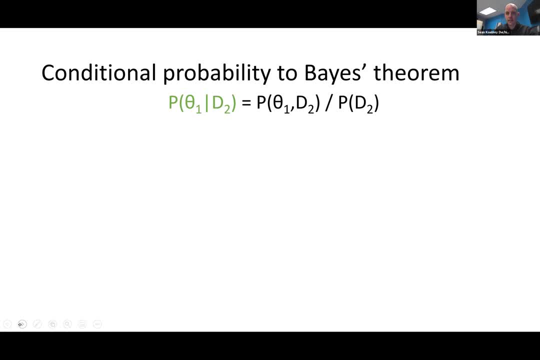 That P of Theta 1, given D2.. That's the intuitive definition of conditional probability. if we just generalize this Now, we're moving away from that table and those specific examples. Let's just think about sets of parameters, Theta, and sets of data, D. 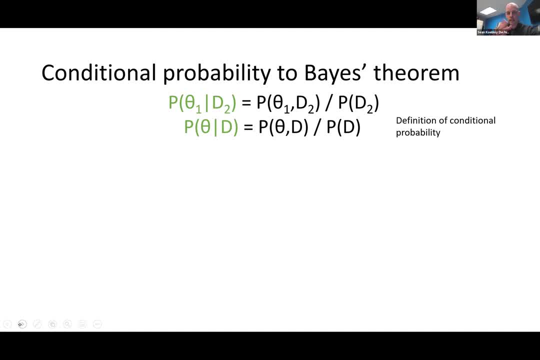 For any set of parameters, Theta. this still holds true. This is the power of this basic logical relationship of conditional probability. Here's the algebra Again. I might be going a little too quick now to follow along, so maybe you can just absorb this and absorb the beauty of Bayes' theorem. 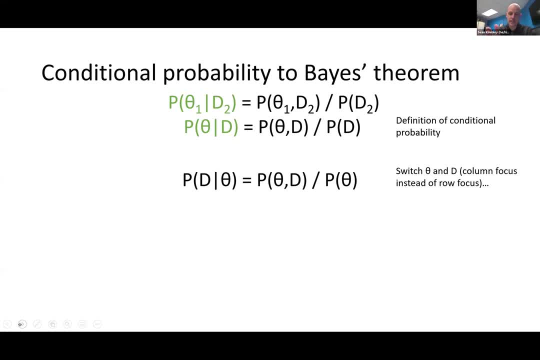 We're just going to switch Theta and D. It's the second question that I asked. You can consider focusing on a column instead of on a row and get this relationship P- D, given Theta equals P of Theta and D divided by P of Theta. 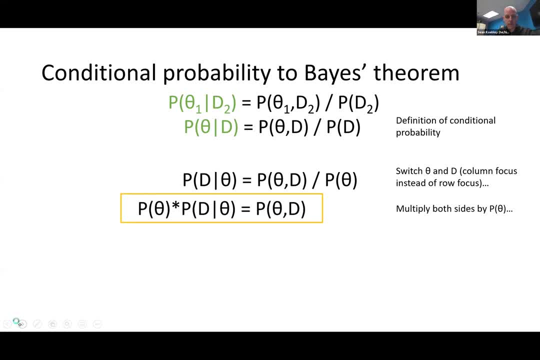 Here's the algebra: Multiply both sides by probability of Theta. We see a common term here, that and term. We can plug that in to your original equation and that's Bayes' theorem. That's as simple as it is. The probability of Theta, or your parameters, given your data, equals your prior parameters. 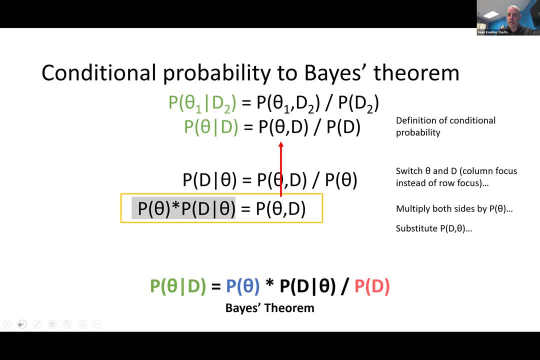 P of Theta times the special term P of D, given Theta divided by P of D. This is where the vocab comes in, and I think it's pretty important. I would write down Bayes' theorem and then write down each of the definitions of these terms, because they do pop up quite a bit. 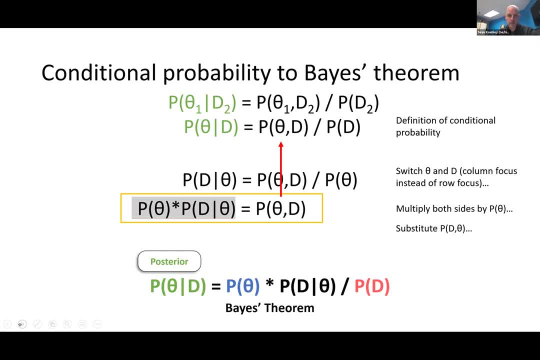 and it'll help you keep your bearings. That probability, that P of Theta given D, is called the posterior. Again, that's our most intuitive endpoints of an experiment. That's our prior. There's no condition there, It's just the probability of your parameters, your naive guess. 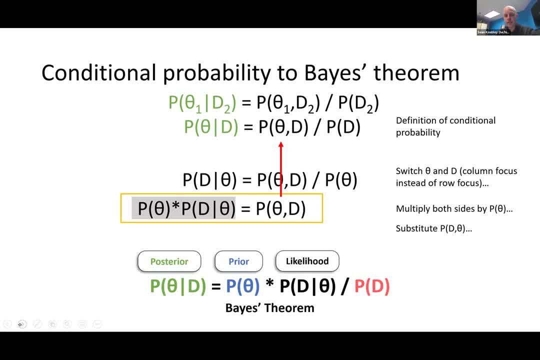 This is called the likelihood, this term probability of D, given Theta, We're going to call that red term marginal data. It's actually got a bunch of different terms. I'm going to call that red term marginal data. I'm a person not a fan of any of them because they're all misleading. 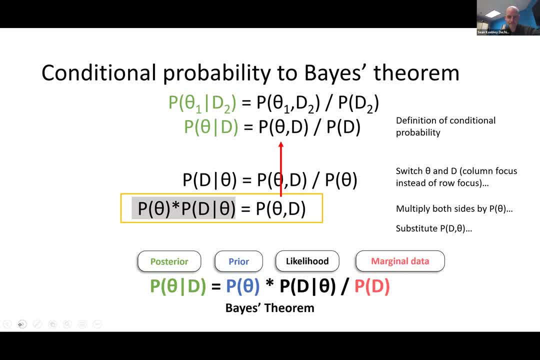 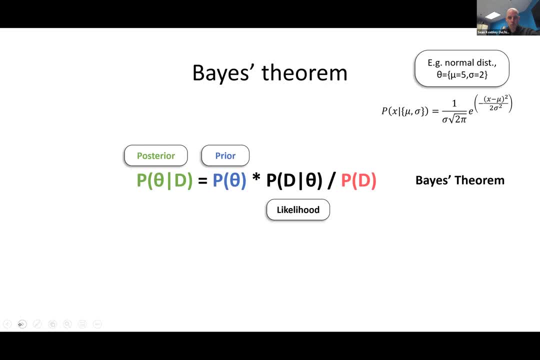 We're just going to call this the marginal data term. Here's Bayes' theorem, and we're going to see how this would work when we actually get some data and do an experiment. For example, say we're considering normally distributed data, Maybe we have the parameters of a mean of five and a standard deviation of two. 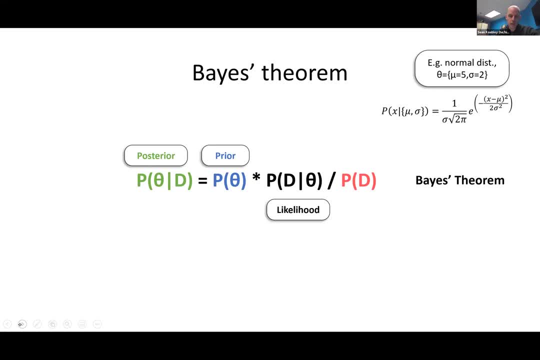 You can see up in the right-hand corner. We know that our equation for a normal distribution or the probability distribution function for a normally distributed equation is this: The P of some term of some number, x, given your mean and standard deviation is as it's written there. 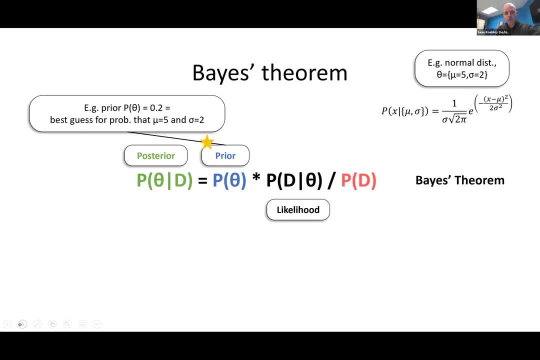 We can find a prior just by using our prior knowledge. For instance, perhaps the probability of a mean of five and a standard deviation of two you think is 20 percent. You think that's a very high probability. Remember, we're talking about probability. 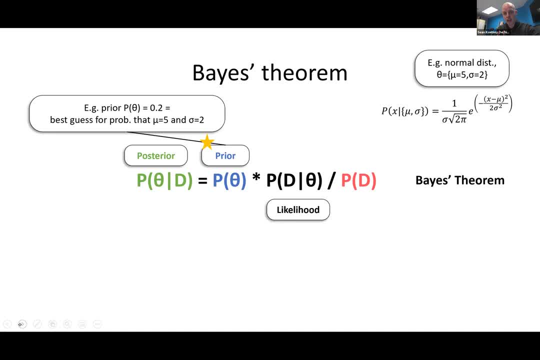 it's got to all add up to one. This would be a very high percentage. You think maybe this is the most likely mean and standard deviation. You can just set that. By the way, what you're actually going to do when you do this is set. 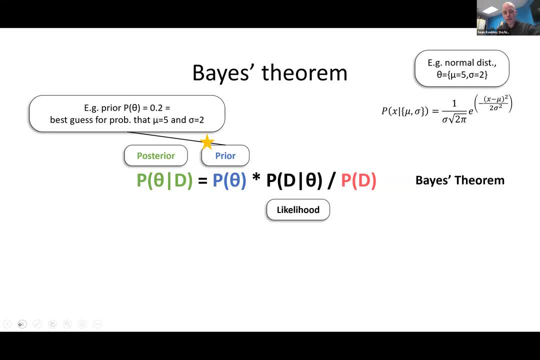 a distribution for your mean and your standard deviation. You're going to say: this is what I think the most likely distribution my means are. this is what I think the most likely distribution of my standard deviation are. You can just use those based on your prior knowledge. 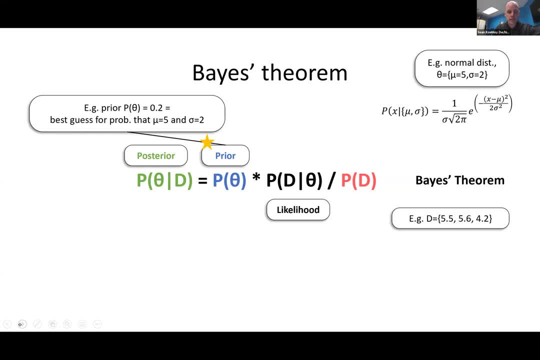 Then there's this likelihood term. Say that this is the dataset. we got three points: 5.5, 5.6, 4.2. What we can do is to find the probability of this data, given our parameters, Pd, given theta. 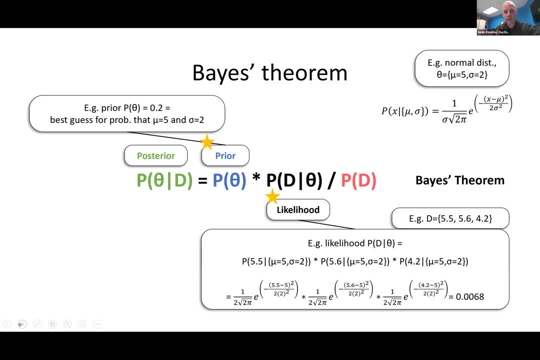 We can just plug it in. Likelihood function is just plugging in your values. If you think back to how we calculate the probability of independent events, and what's the probability if I get three heads in a row and I flip a coin? 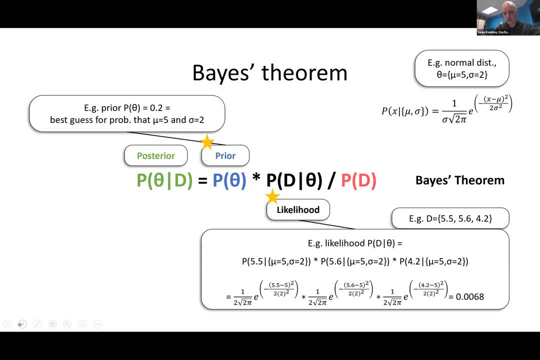 you multiply the probability of each case. That's how you find the likelihood value. You multiply the probability of each individual data point. In this case, you can see here I just plugged in the values of 5.5, 5.6,, 4.2.. 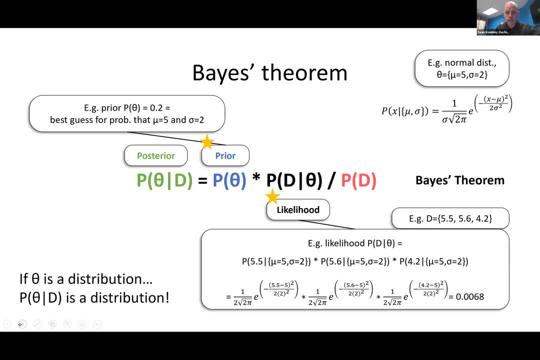 Very easy for a computer to do this. You can get a value there of 0.0068.. There's what I was saying about your parameters. If your parameters are a distribution, then your posterior is a distribution, which is a very interesting thing. 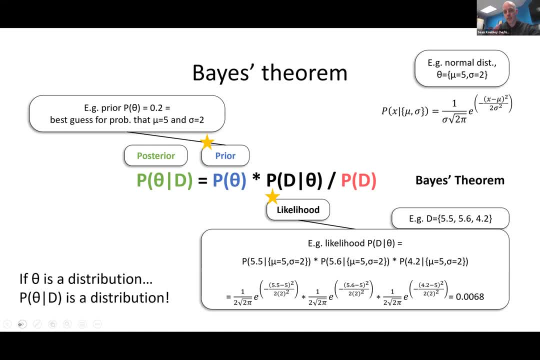 We're not just getting a single P value. You're going to get a distribution of your most likely means, your most likely standard deviations, instead of just a single value. Then you can use that to make your inferences. But I just want to hit this home. 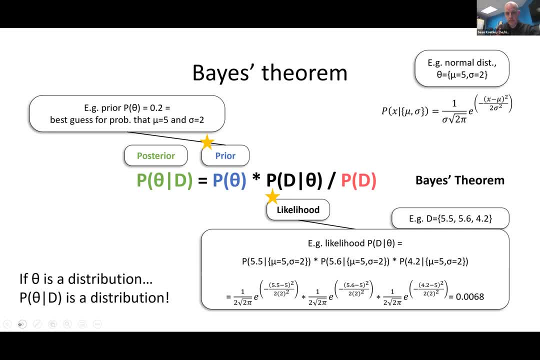 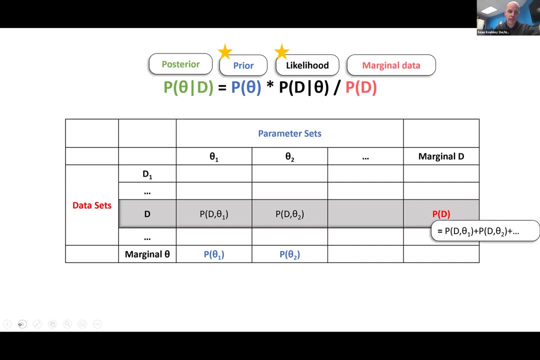 I starred the prior and the likelihood, because we can find those, Given that we have some prior knowledge of our data. we can find those two values. You can actually plug in numbers for those. It's that last term, that marginal data term, that's been the trick. 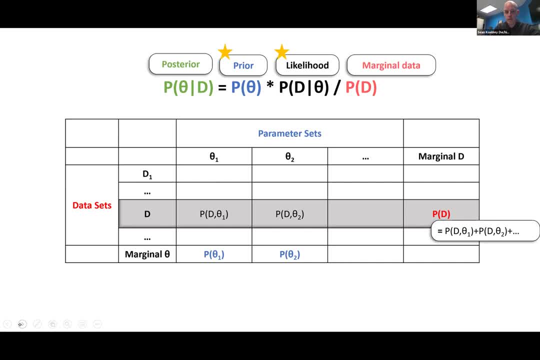 This is the reason Bayesian statistics hasn't been used in the past is because we've got to include that marginal data term. You can see how I just laid this out in a general table. You've got to include all possible datasets, which seems like an impossible task. 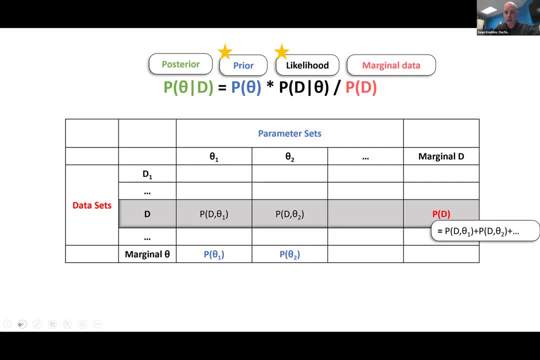 There's ways we can massage this term to make this possible. That P of D term is just the sum of everything in that row. But if you remember that P of D and theta, we can actually do that. Look back to that derivation slide and see that we know an equivalency for this. 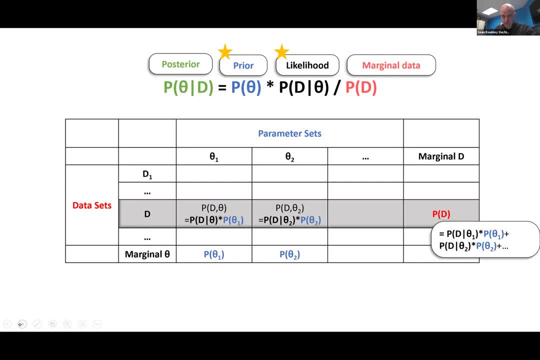 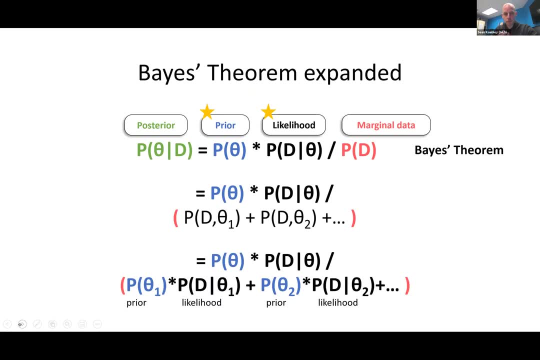 That's equal to our likelihood times. a prior, Actually P of D, is just the sum of all possible priors times, the data given those priors, It's the prior times. the likelihood for all possible priors Still seems tough because you have. 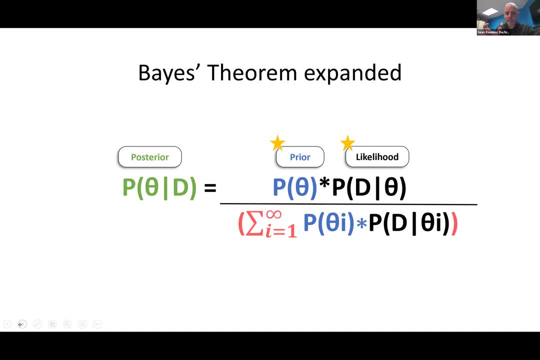 to sum all possible priors in the denominator. there You have that infinity term and I probably could have used an integral there instead of a sum term. The question is, those i's should be subscripted. I'll fix that when we go back to this. 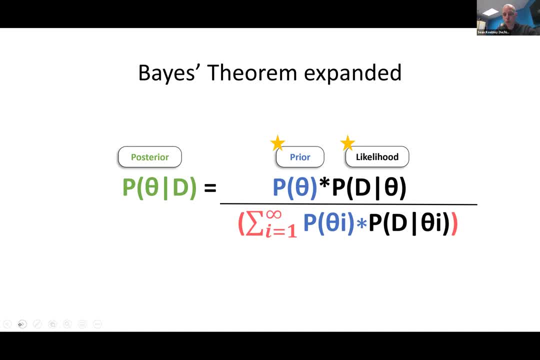 But that's the trick here. Can we find some way to test all possible sets of priors, or do we need to Anytime we get into infinity or close to infinity? you should be thinking maybe this is a good job for a computer to try to. 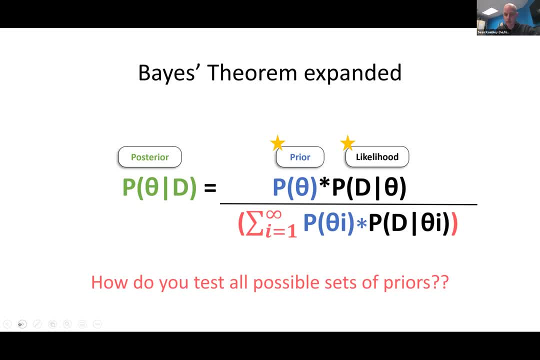 get close to the answer in an approximation that is close enough. In fact, that's the way to solve this, and that's why Bayesian statistics has become more possible. The integrals in the bottom of this equation were impossible, except in some special cases. 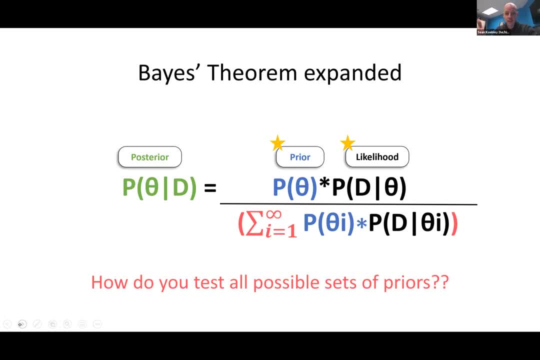 before. they're still impossible to analytically solve, But with computers we can computationally solve them. We can do enough tests where we get close enough answer to this. So that's, that's the key, And maybe I'll go through this real quick. 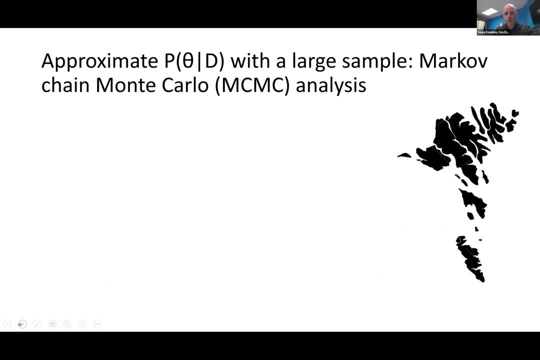 In order to do this with a computer, using something called the Markov chain Monte Carlo analysis. it's a really cool and simple technique And I love this example. Say, you want to visit an island a number of times proportional to its population. 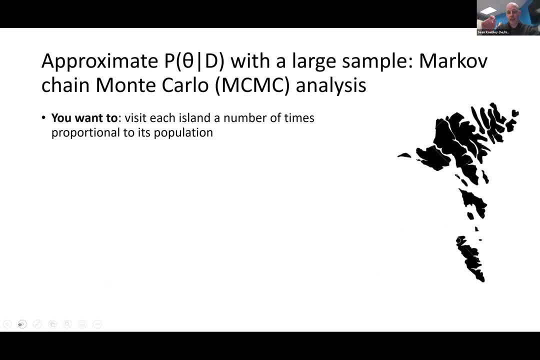 You're a politician and you want to visit every single one of your constituent islands, and everyone has a different population. Problem is you don't know how many islands there are or how many people live away on the faraway islands. Each one of those islands is different. 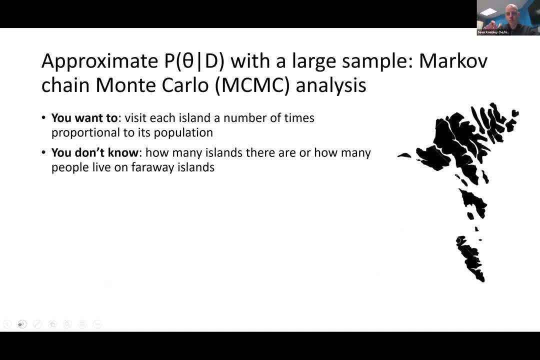 They have a different parameter set And the number of people is the likelihood of that parameters. You might have an infinite number of parameters, with each one having a different likelihood. That's the case we're considering here. What you can do is find the population of adjacent islands. 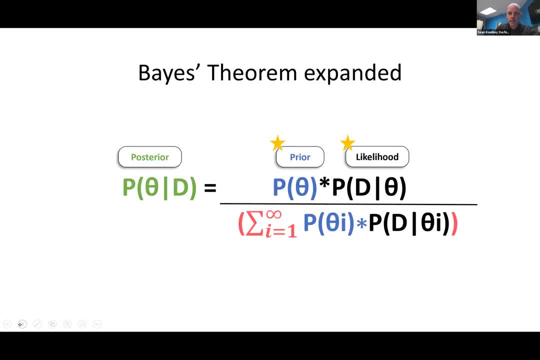 So if you go back to our calculation here, remember we can find the prior and we can find the likelihood, So we can find the property for a single island or a single case, we can find the posterior, but we just can't find, you know, the that infinite. 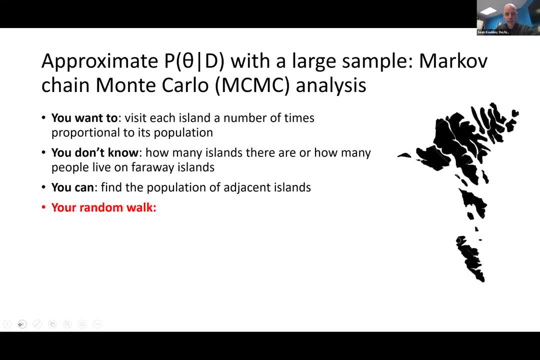 case. So what we're going to do is take a random walk, And then that's what this money, Markov chain, Monte Carlo analysis does. It's doing a random walk along these islands. You randomly choose an adjacent islands, Um, I you find the population of that, which is, uh, the likelihood times, the 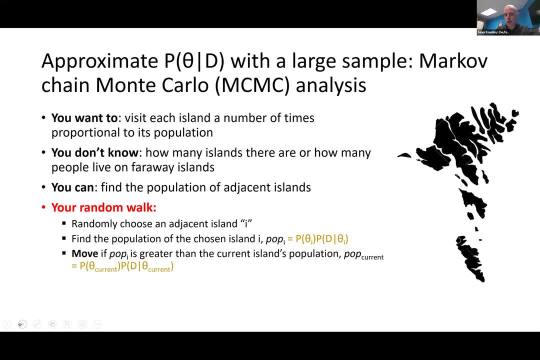 prior and you move If that population is greater than the current islands population. So you move to that next parameter set and you stay if populations less and you choose a random number and it's greater, uh, than the population of the adjacent Island divided by your current population. 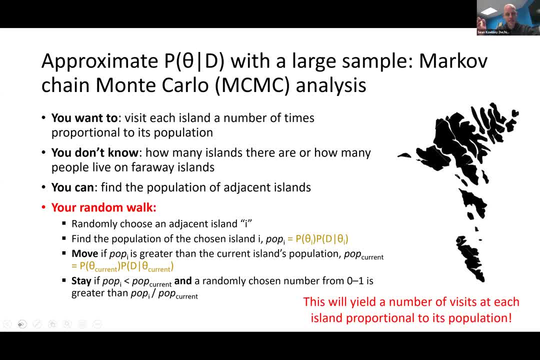 So, again, these details don't really matter, but I want to give you a sense of how simple this is. because we do this thousands and thousands of times, You're actually going to yield a number of visits That's proportional To the population of each Island. It's just a really cool concept. Um, so this is a way to get. 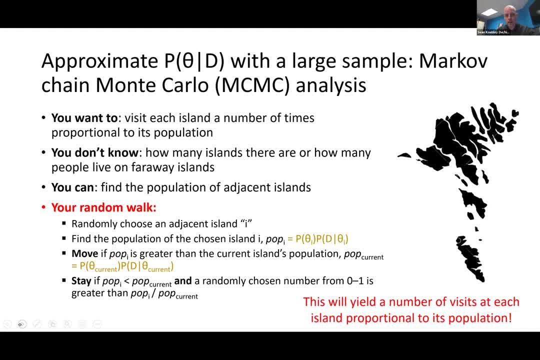 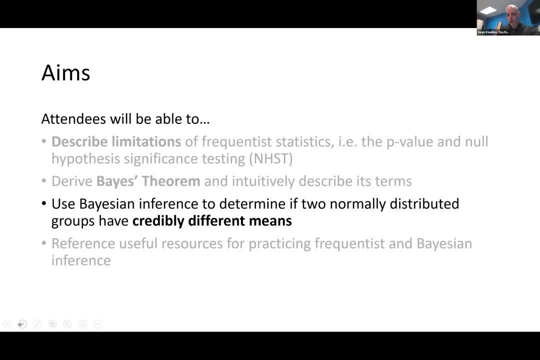 a sense of that posterior distribution, um, from using this, this, these computational tools. So now that we've kind of got a sense of the vocab and hopefully an intuitive sense of of how we got there, we're going to use Bayesian inference to determine this classic case You got. 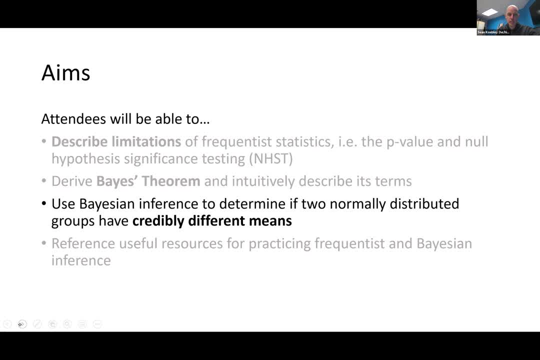 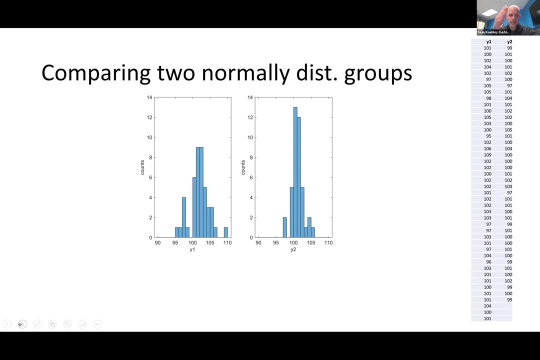 two normally distributed groups and see if they have different means. Okay, So here's the data. Uh, we've got why one and why two and you could see the histograms here. It looks like the means are pretty close. Um, you know they don't. this data doesn't have to be normally distributed by 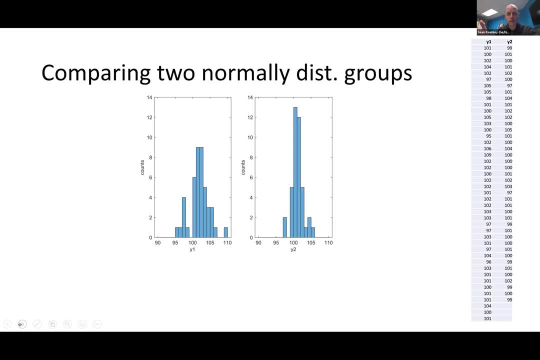 the way you would just, um, you know, use a different function just to describe the shape of the data. In this case, I would say they do kind of both look normally distributed. So I would, I would probably use a normally normal distribution, And we're going to ask, given this data, 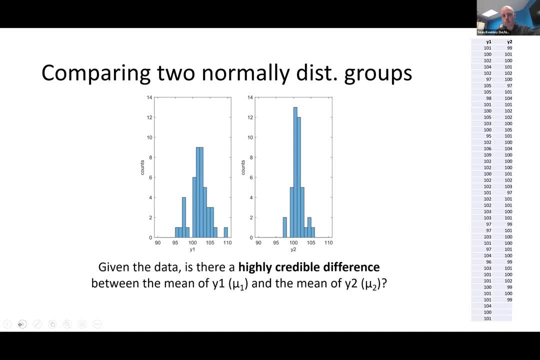 is there a highly credible difference between the mean of Y1 and the mean of Y2?. So again, think about the way we're phrasing this. This is exactly what we're going to find when we find the posterior P of theta given D is. we're going to find those parameter values. 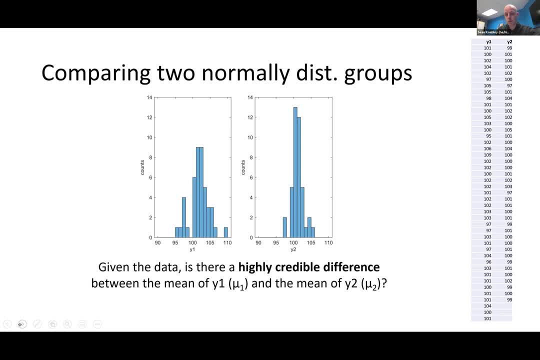 mu one and mu two, given the data? Okay, So this question is perfectly aligned with Bayesian statistics, And another way of phrasing this, or maybe something else added onto this, is asking: is zero included amongst the most credible values of mu one minus mu two? So is your difference? 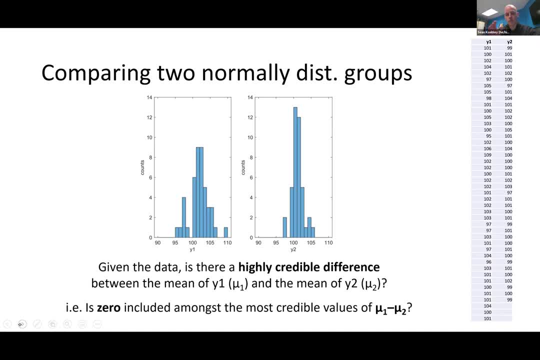 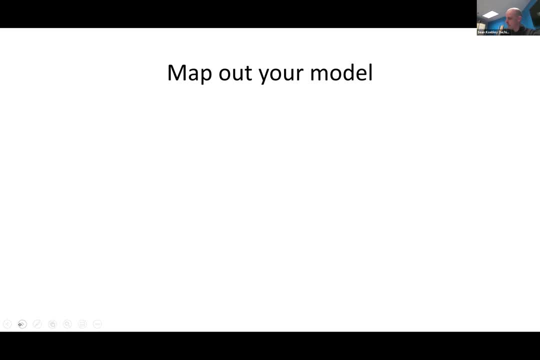 between the means is a, most is is zero, one of the most likely values that you're going to find. So what we're going to do- this is maybe, if you've got another piece of paper, I'm going to show you that this is a really important step- is mapping out your model. 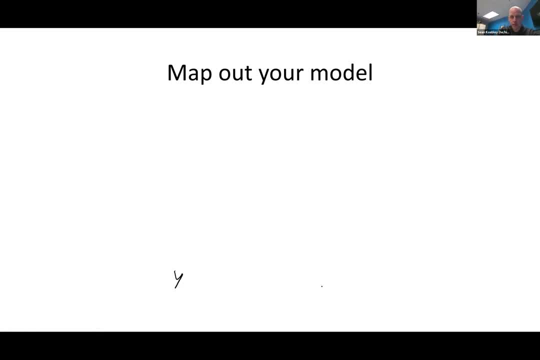 Okay, And here's how we're going to do it. We're actually going to. we're going to start at the bottom of your paper. We're going to start with your data, You know Y1 and Y2.. Again, that data looked normally distributed to me. So I'm going to say: 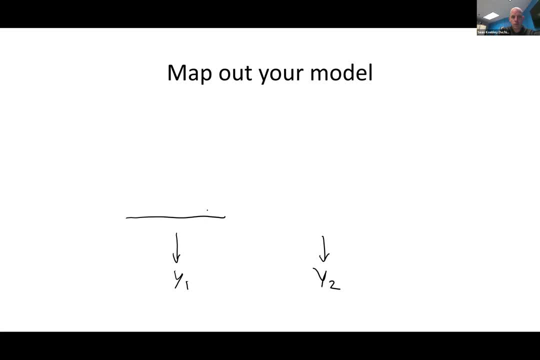 that that data were derived from two normally distributed populations. Okay, And I'm just going to list out the parameters included in those distributions. So each one has a mean and each one has a standard deviation. Okay, Now we define our priors. This is where we kind of get away from this. This is what's really powerful about Bayesian. 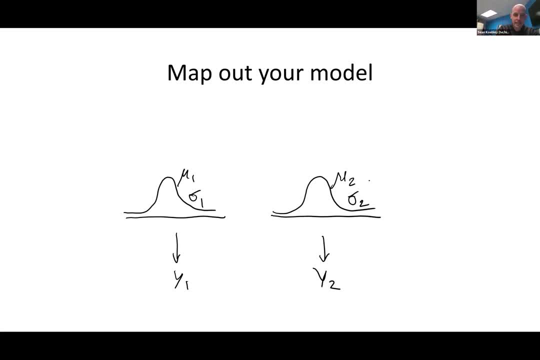 statistics is you get to define your priors. Say, for my mean, you know, I think it's a pretty good assumption that your mean is also that if I, if I took multiple tests, you know this, or yeah, my prior knowledge is that this would. the mean is also normally distributed. 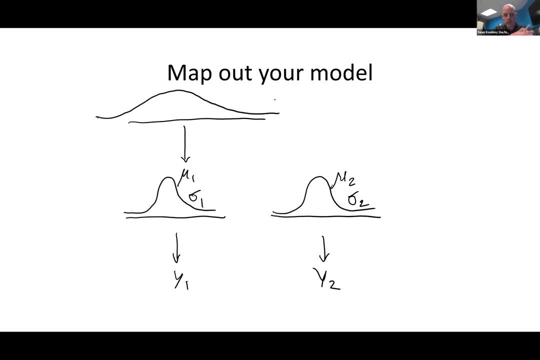 Maybe it's a little broader, Maybe there's a lot of different possibilities for that mean, So that prior distribution has a mean and a standard deviation. I'm going to call that M and S. Again, this is the distribution of prior means that are the most credible. So my most credible. 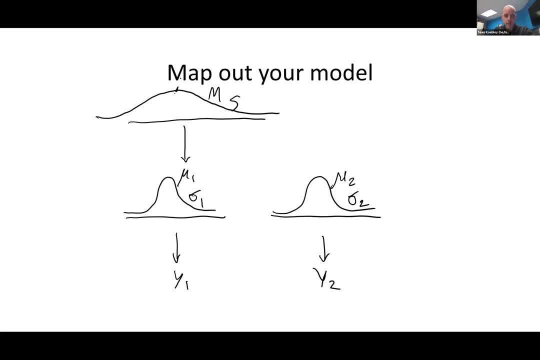 mu one is right at the top here, but it's still possible, maybe in my mind or my initial guess, that the mean could be something much farther. So I'm going to start away from that. This is just my prior guess. Okay, You can do the same thing for. 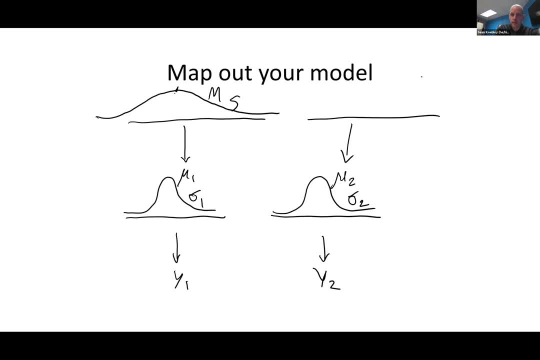 every other parameter. You can give priors for each one. Maybe you can use the same values M and S. Maybe you have no reason to believe they're coming from different distributions. You can do this, and I think the main point here is that you want to be transparent with this, Whenever you're. 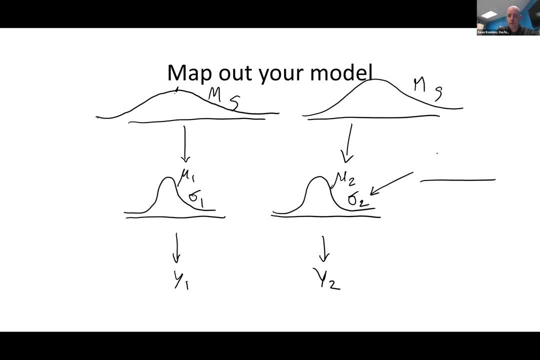 publishing your paper or discussing how you're doing this experiment, you need to lay out exactly how you did it, And that's easy because you can just show exactly what you used for your priors. For my standard deviation, I can't go below zero, So maybe I'm using some other distribution. 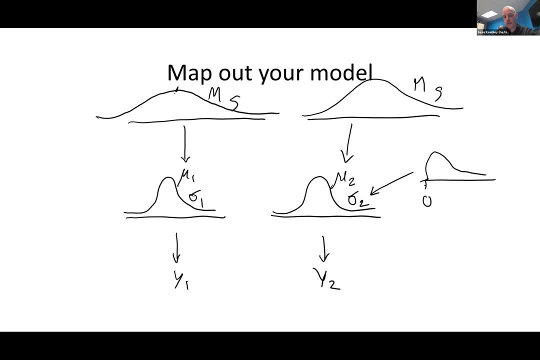 in this case a gamma distribution that just tails off to infinity but doesn't go below zero. And same with my sigma one. I'm just going to go from zero and it goes to infinity. Okay, Not really important, I'm just going to go from zero to infinity, Okay. 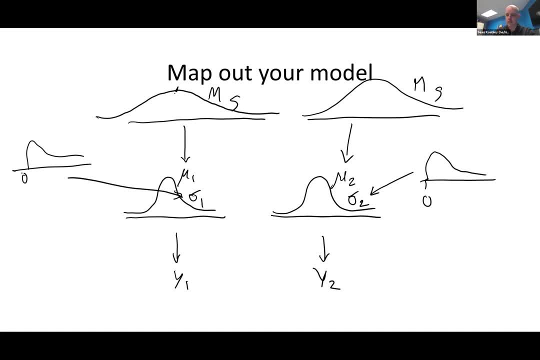 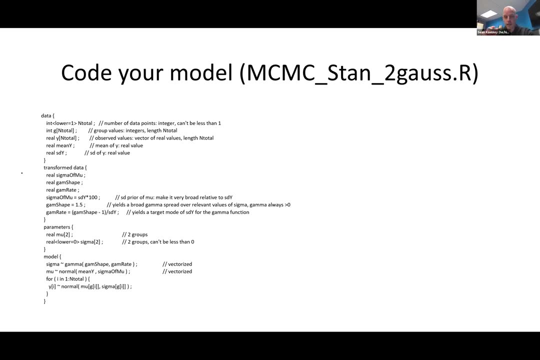 Not really important what those are, because, again, you can choose those based on your best knowledge of the situation. So that's my model, And what you do next is turn that into code. So, this code that you're seeing, I'm going to give you this, this whole file. 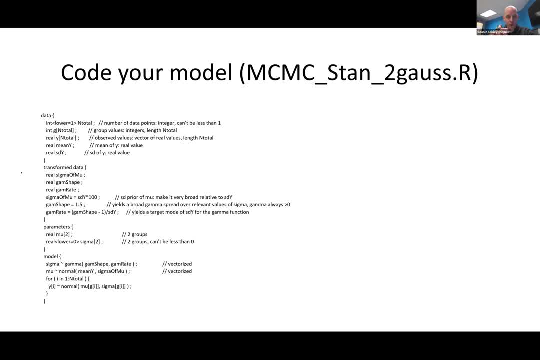 And you know I commented it out as best I can. Don't worry about looking into it right now because we're going to move on in just a second. But you know, I just want to maybe impress on you that it's not that complicated. 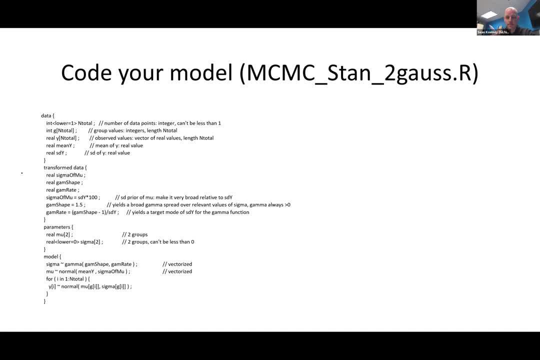 There's really not that complicated. There's not that many lines of code here And there's a lot of examples in the resources that I'm going to give you on how to write this. This is in Stan. It's an open source language, So you can. there's tons of documentation on how to write in this language. 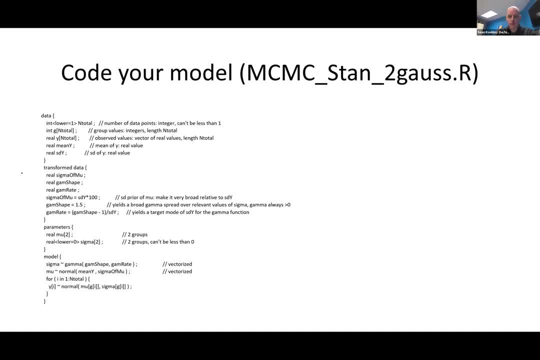 I've already done quite a few different things with this. It's very flexible, But I will say this is probably the trickiest part of dealing with Bayesian statistics. So you have to run the code, You have to figure out how to code this and make it work. 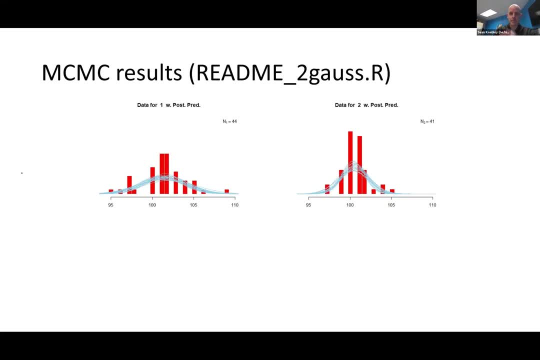 So when you do that, You plug all this in And again I'm giving you the file here That you can refer to and you'll see exactly how to produce these plots. but I'm showing our data in red and then 20 very likely parameter sets that are plotted. 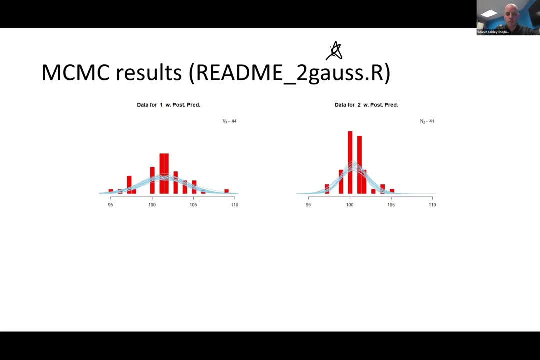 So these are kind of the 20 most likely. theta one and sigma one or sorry, mu one and sigma one are so most likely means and standard deviation. So you see they fit the data pretty well. Really Powerful part is that I get back from that random walk distributions, the posterior distributions of each one of my parameter values. 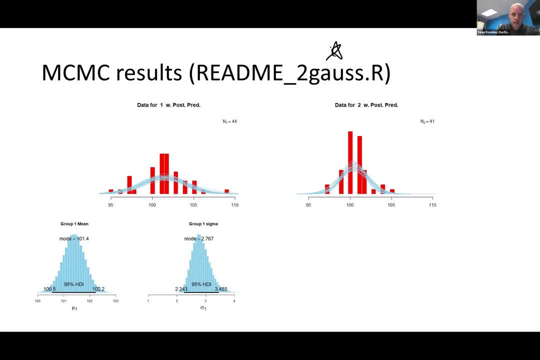 So what I'm seeing here Is is the mean mu one and the standard deviation sigma one for my Bayesian inference test, And these are the most likely means and standard deviations given the data. This is p theta, given D. I just These. these plots are beautiful. I think they're absolutely beautiful because even a confidence interval. 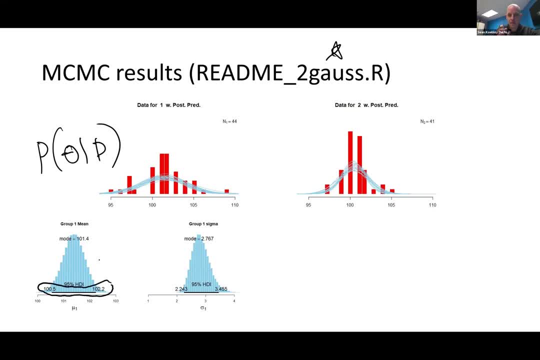 It's just going to give you down here what you're seeing. there is the 95% highest density interval. Those are kind of the 95% most likely means conference interval is going to that's. that's basically, you see, with the confidence or just the bar. 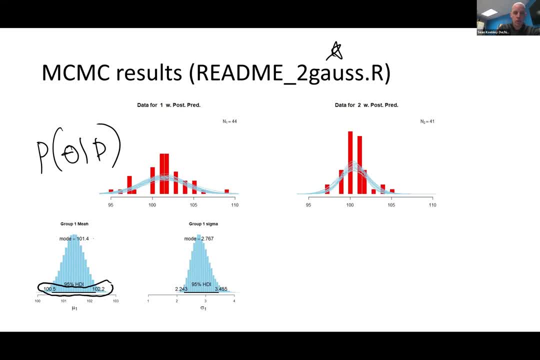 Here what you're seeing is the distribution. So you're getting a mode, You're seeing the most likely mean value and you're seeing kind of how that, how those most likely means are shaped, same with your standard deviation. and of course you get that for your second distribution as well. 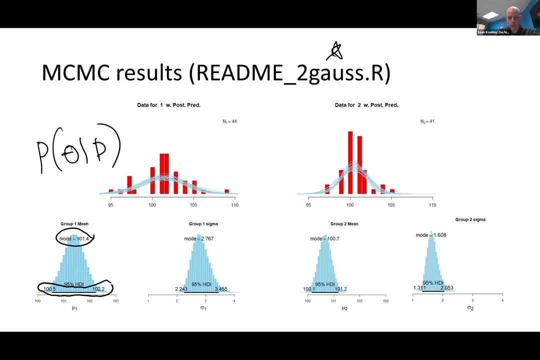 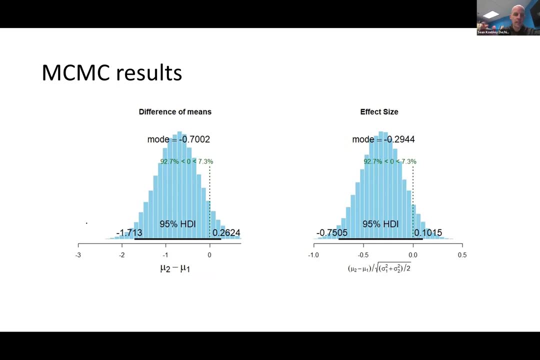 you see a different distribution of means distribution, different distribution of standard deviations. so what you can do is, for every single one of those priors- remember we tested to get this data. i think there's 50 000 tests that i ran- every single one of those, you can calculate the. 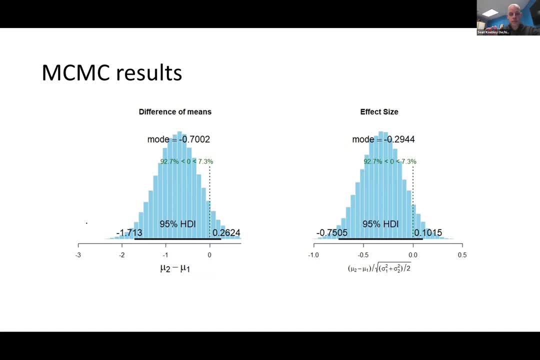 difference between mu 2 and mu1. and you can ask: is zero among my most credible values? and look, look at that zero is within your most credible values for mu2 minus mu1. so we can say that there's really no credible difference that we can see between these two populations, because 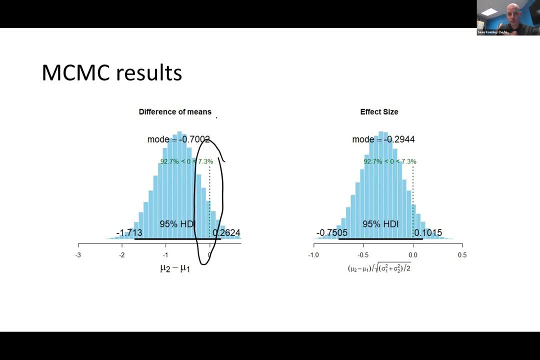 or between the two means, because zero is within that 95 percent highest density interval. you can also look at the effect size. you can do whatever you want. you just get a huge table full of those 50 000 values for every single prior. you've got your the posterior. 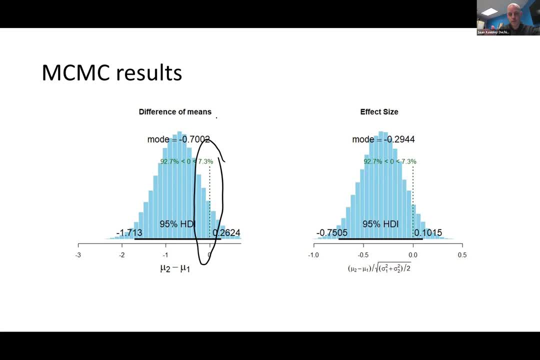 you know values for every single one of those parameters. very powerful stuff. so there you go. the conclusion is that yes means the. the two groups are not credibly different is how we would say that try to stay away from that word significantly, because it has so much import. 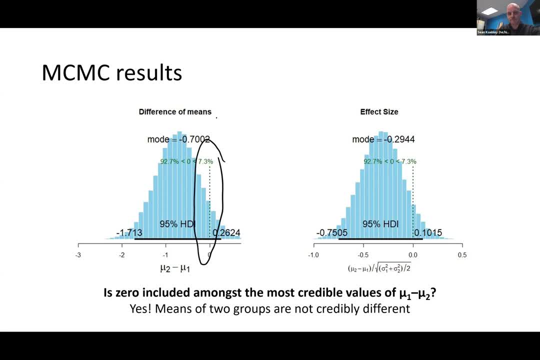 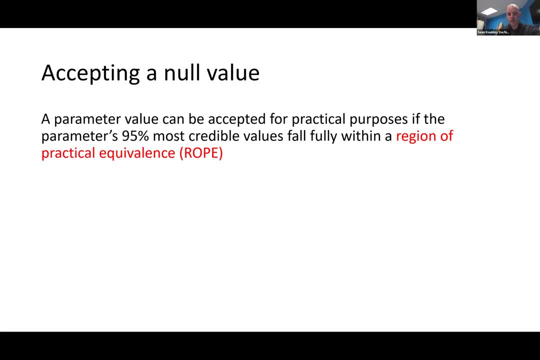 in a null hypothesis significance testing. so one of the great things about Bayesian statistics, too, is that you can actually accept the null value because you've got these, these, these distributions of your posterior parameter values. you can treat these as you might be in there, in the most intuitive. 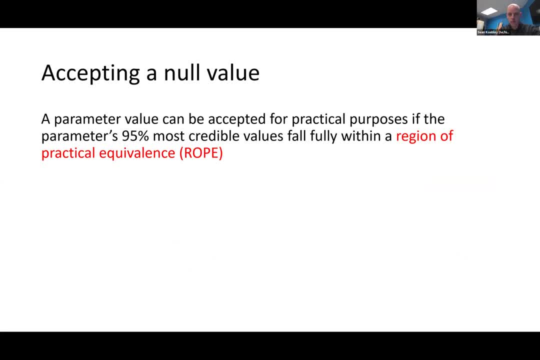 way that you can think so. for practical purposes, you can accept a null value if it falls within a region of practice equivalence. And again so here's an example of this: Say that our null value is that the mean is 101 for my group one. And say that my region of practical equivalence is 101 plus or minus two. 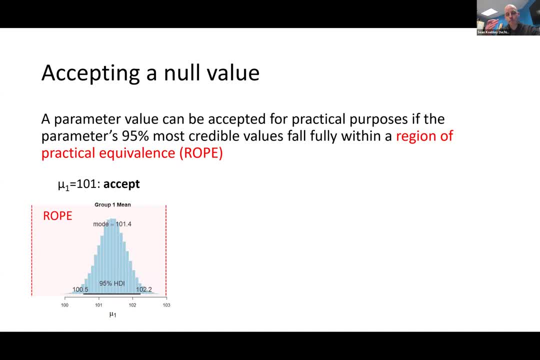 Now, how did I choose the width of my rope? That's again based on prior knowledge and it's transparent. You have to say why you chose the width of your rope. I actually just published a paper where we use ropes in our analysis and we actually used an ROC curve. 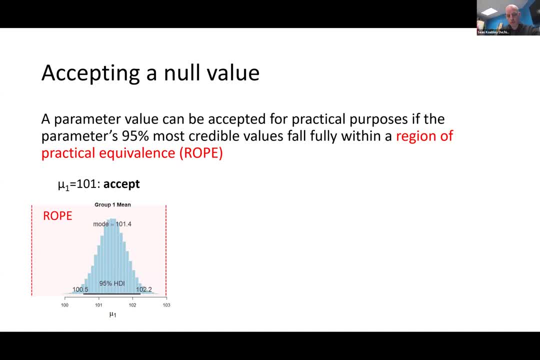 analysis, if you're familiar with that, to determine the width of the rope. So we looked at prior data or preliminary data and said, okay, based on that, we think this is how wide a rope should be And if the 95% most credible means are within that rope, we can say, for all practical. 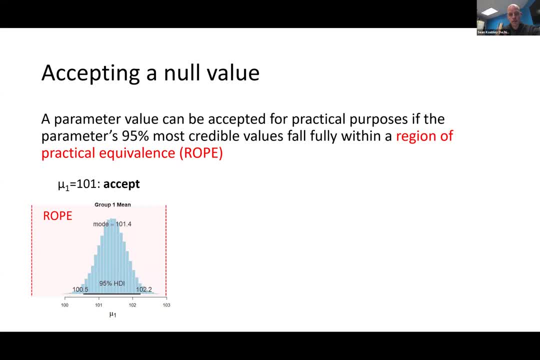 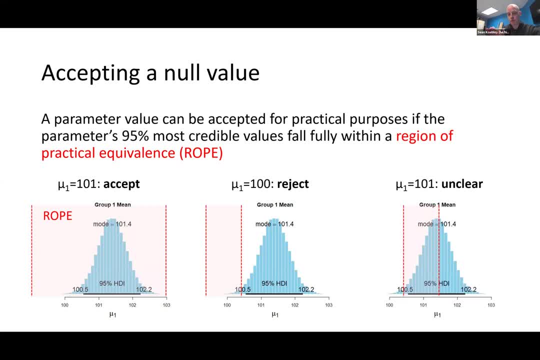 Maybe the 95% value straddles the rope And part of it is inside, part of it is outside And you would say, all right, we can't really make a conclusion based on this test. So again, you've got a lot of freedom to work with how you define your test And because your values are intuitive. 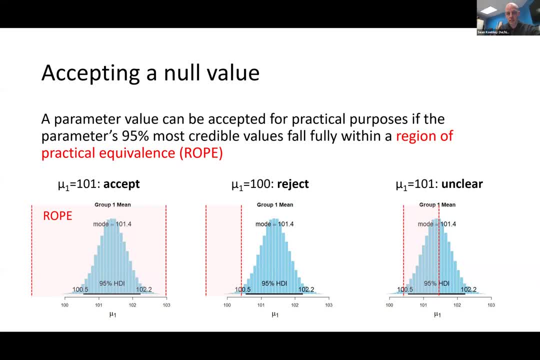 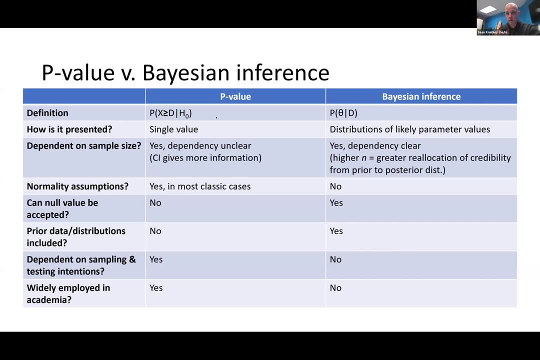 you. you know, I think it's a lot more powerful the results that you get. So finally, last slide here, I just want to do a quick comparison between the p-value and Bayesian inference. Those are the definitions up at the top there And you can see. you know, for me the Bayesian 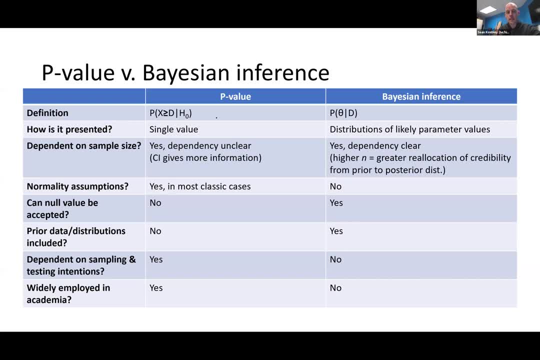 inference, the posterior, the p of theta, given d. it's much more intuitive. They're presented very differently. p-value is a single value. Bayesian inference: you get distributions for each one of your parameter values. So, depending on sample size, both are It's much more unclear. 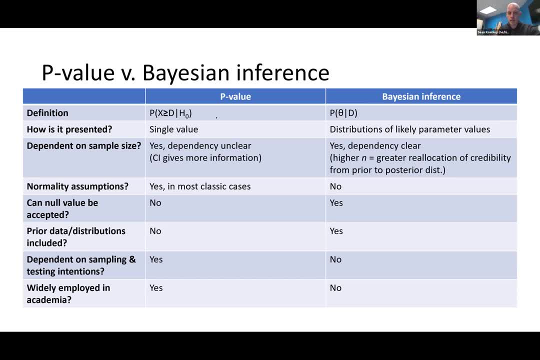 with a p-value what the effect of that population is. Are there normality assumptions In most cases- classic cases- in the p-value? yes, No Bayesian inference: you just decide what your distributions are And you're transparent with those decisions. Yeah, Can null value be accepted? Yes, it can with. 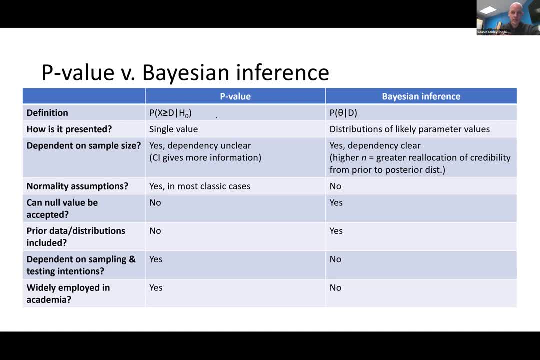 Bayesian inference- Prior data. yes, you can do with Bayesian inference Dependent on sampling. no, not with Bayesian inference Widely employed in academia- not yet. So that's where we are, And here are some great resources. This is what I use to learn all this. 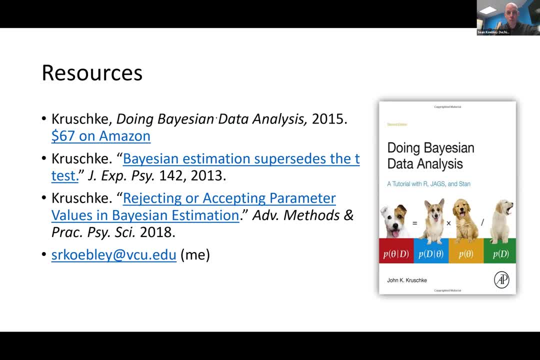 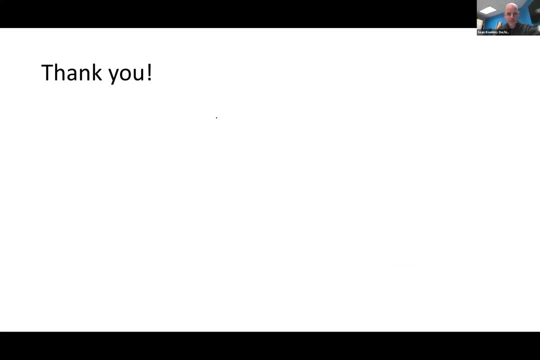 stuff. that textbook is fantastic And I'm willing to help if you want to give this code a shot with your own data. So with that, thanks, And we have a little bit of time for questions. Happy to answer these And, again, everything's going to be online So you can try this out for yourself. Any questions? 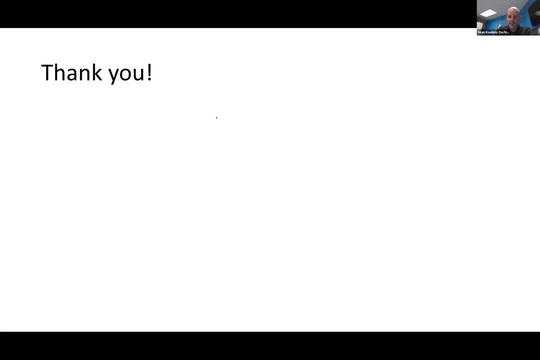 I know it was a lot. I should have done a poll or something. I want to see how people feel. It's hard with Zoom to see where the audience is. Hey Sean, I have a question about R and computers. Is there a particular computing need in order to be able to do R? Because I've talked with some 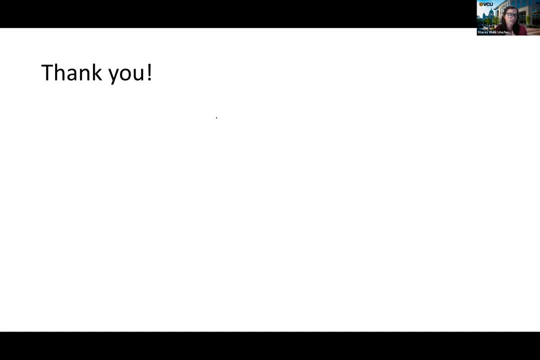 folks who have older computers, And then can you speak to that a little bit. Sure, Yeah, I think it really depends. So the data set that I worked with I think we had like 1.5 million points of data And that took me a few days with a relatively fast computer to run all that.